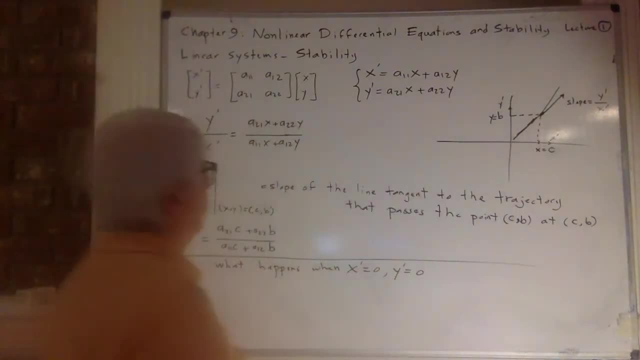 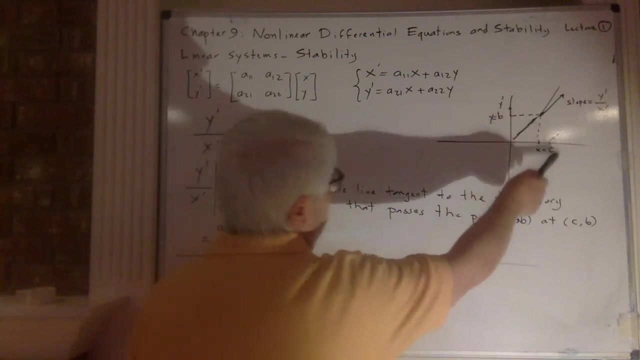 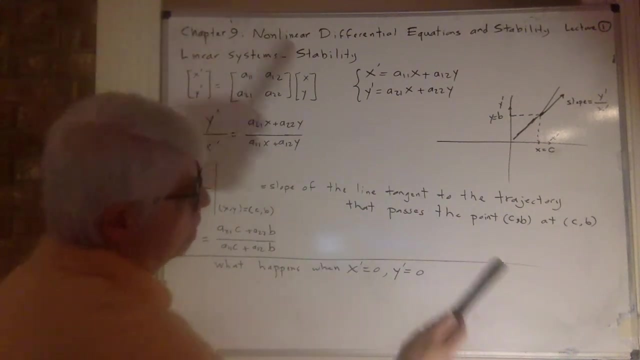 at any point x, y. So if x is c, for example, y is b. at point c b, the x' is speed on x-axis and y' is speed in the direction of y-axis. So y' over x' will be tangent. or 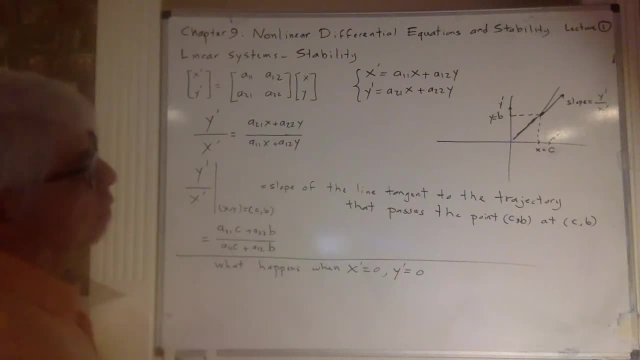 speed In fact, or let's say velocity in fact, Velocity in that direction, when it goes in that direction. that's the trajectory. It's like an object is moving on that trajectory, But anyway. so at point c b we get this. So this is in fact slope of the line tangent. 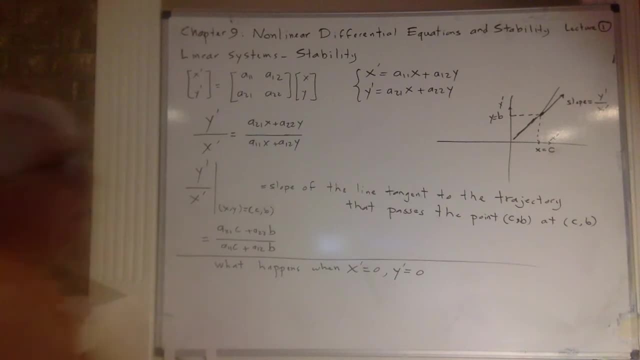 to the trajectory that goes through point c b, at c b- And remember, we have infinite trajectories, In fact many, many, many trajectories, uncountable trajectories- and one of them goes through point c b, And at that point the slope of the line tangent is, in fact, y'. 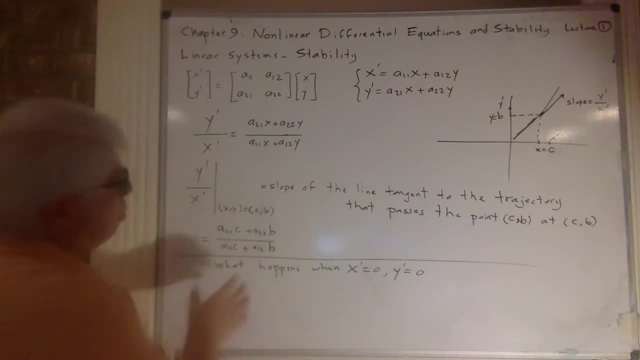 over x' It's for every point of a. at that point is this number. Now the question is: what happens when these two are zero, which means that it stops, So the particle has stopped. So when or where does this happen? Let's look at this equation up here. So the question: 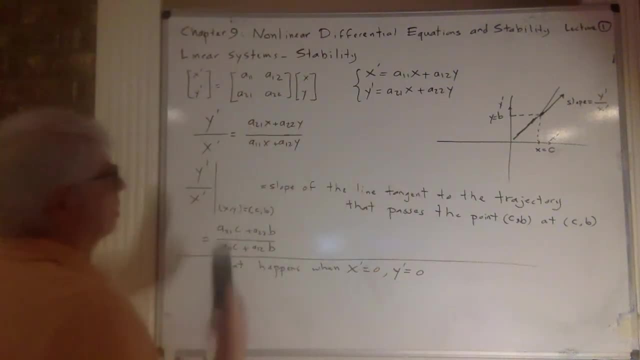 is where? at what point does this happen? Okay, let me erase this and look at that. So, when x' is zero and y' is zero, this gives me a simple system of equations. in fact, There is this thing: a11x- a12y zero and a21x- a22y zero. So this is in fact this. 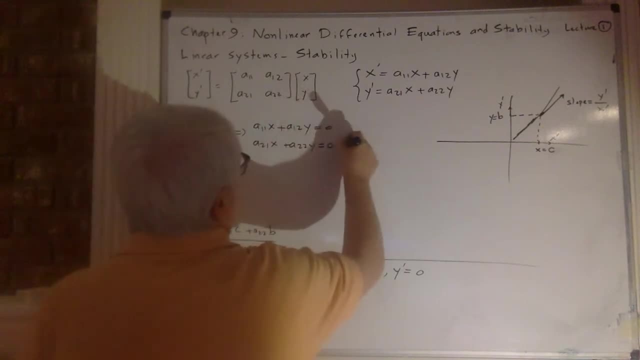 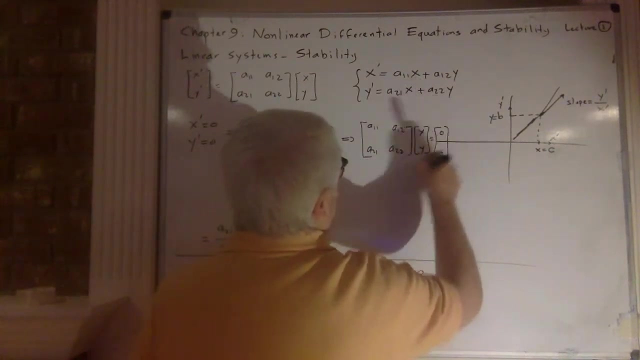 matrix a11, a12,, a21, a22, times xy, and that is zero, zero. Now I'm assuming that in fact this is the matrix. Okay, Okay, Okay. So let's assume that this matrix is not singular, so its determinant is not zero. 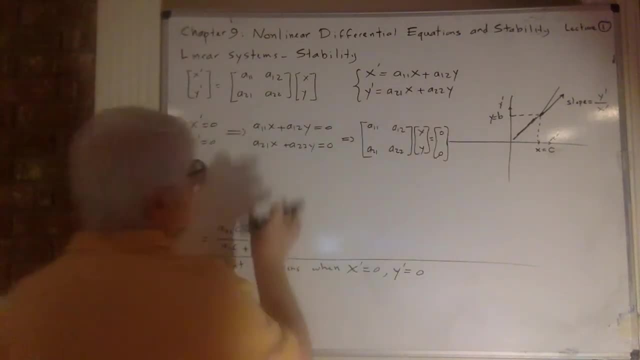 If this matrix is singular, its determinant is zero, then the second equation is the same as the first equation, So let's assume that they are not the same. Okay, So this gives me just one solution. If that happens, it has just one solution. 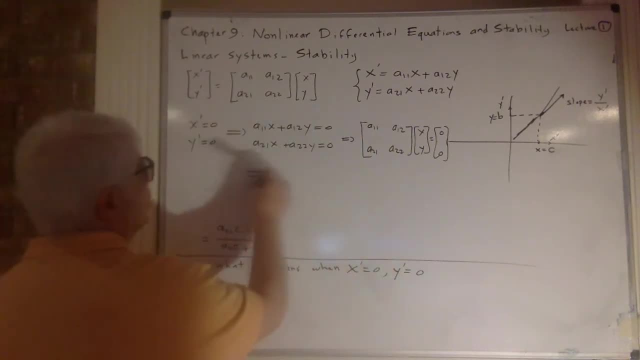 and that is in fact zero. And that is in fact point: x zero and y zero, which is the origin. Okay, So at the origin, at the origin, y' is zero, x' is zero, so y' over x' is zero over zero. 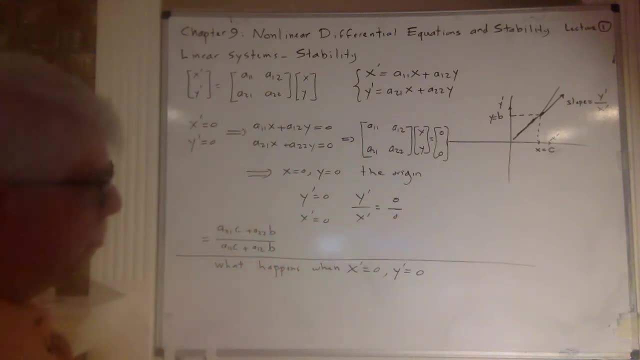 So, which means that it's basically undefined, because that can be just any number. So what? what does it mean? Well, the trajectory has slope, undefined, slope at point zero, zero. Now we know that the trajectories, in this case at least, they tend to just go towards. 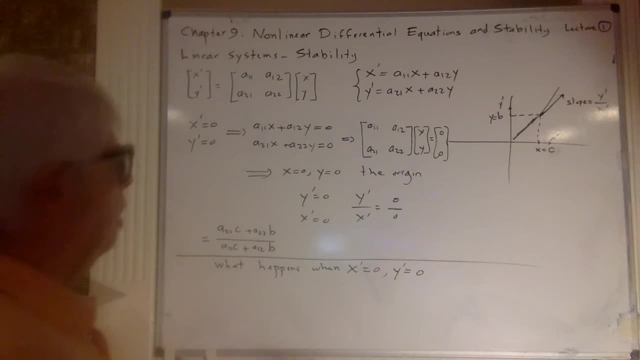 point zero, zero, zero. What happens? I can ask this question: do they really reach that point? The answer is no, Nope, they. they are not. No, no trajectory ever reaches that point. They get closer and closer, and closer and closer, but never reach that point. 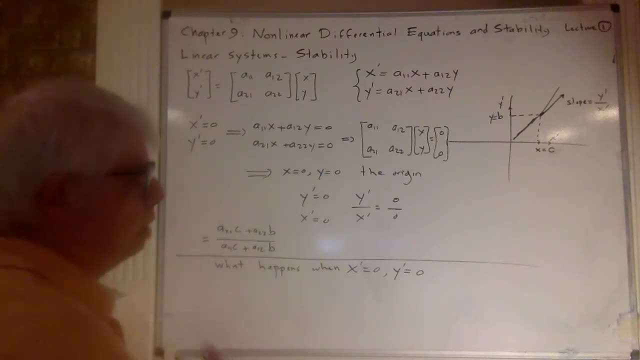 That's in fact. we will see why this happens and what really that means. So this point, at which the slope of the line tangent to a trajectory that never passes through that point, in fact, is undefined, that we call a critical point. 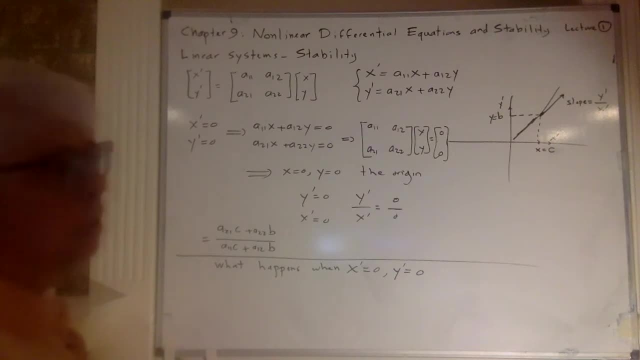 So a critical point is where the slope is not defined, in a sense. And since the slope is not defined, and if the trajectory reaches that point, then there's some slope right, Or if that continues, then it has some slope, So the trajectory never reaches that point. 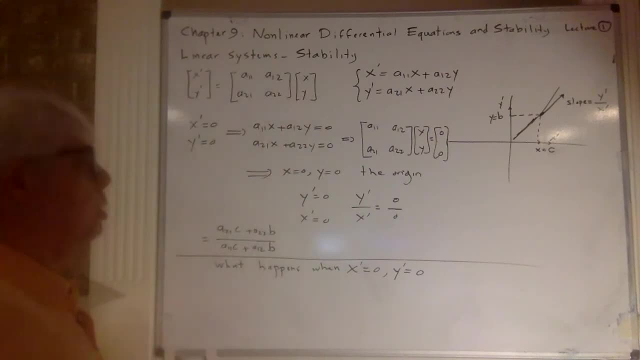 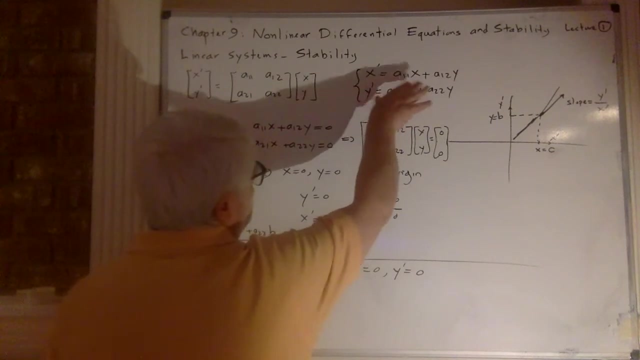 It goes round and round, maybe it gets closer and closer and closer and never reaches that point. So that's called a critical point. So for a linear system, critical point is basically a point zero, zero, And I'm just assuming that these two equations are not the same. 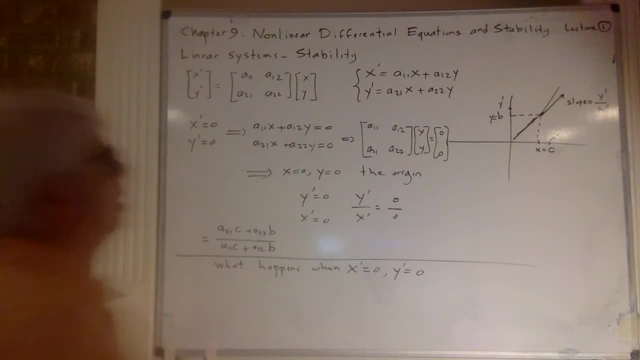 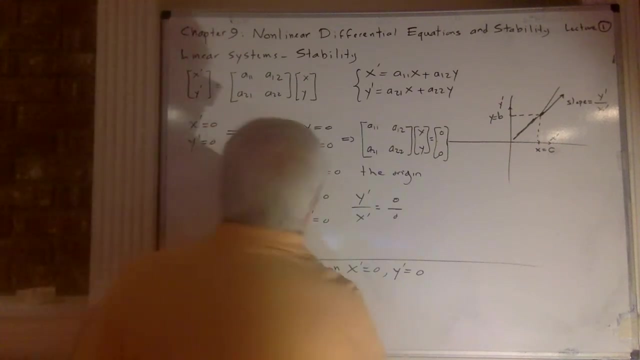 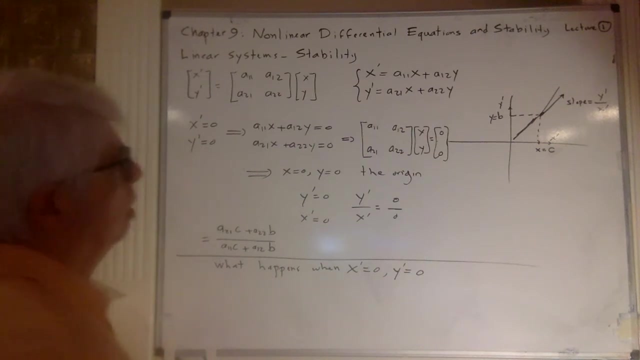 Assuming that those two equations are not the same, then it will always be zero, zero. So let's start with an example, Let's see what happens And I will graph some functions for you here, like x and y. I will find them and graph them for you. 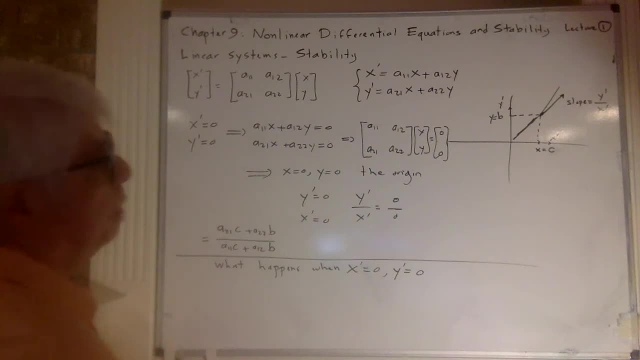 And I will graph the trajectories in the face plane. That's x, y, that's called the face plane. So let me- I have discussed this before, so let me- erase this thing and start with an example. I have two parts for you. 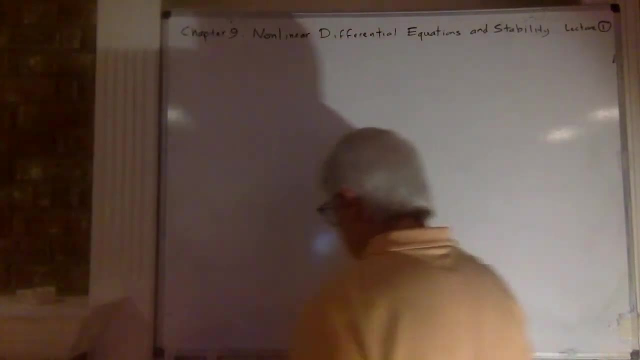 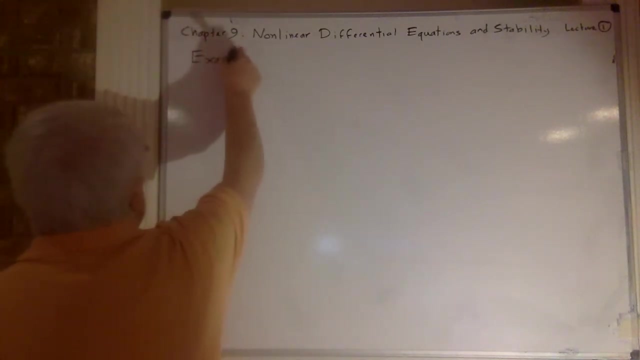 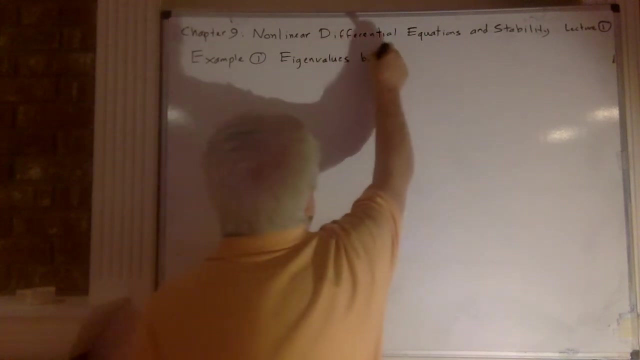 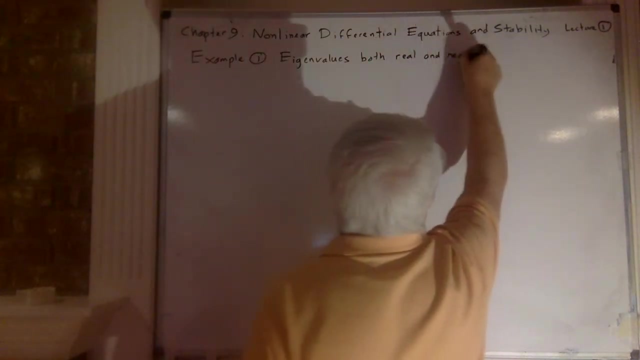 I have two parts for you. Now I call this eigenvalues. I have two parts for you. I have two parts for you. I have two parts for you Both. Let's say real And negative. so let's assume that they are distinct. 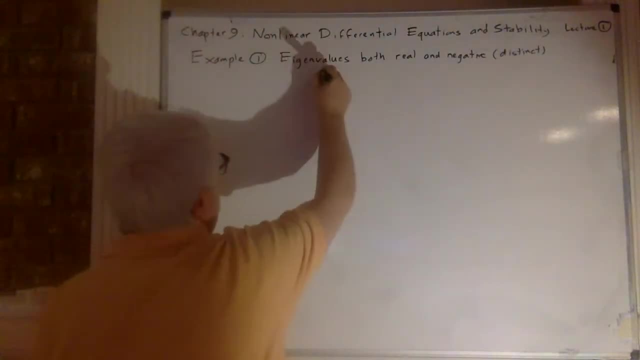 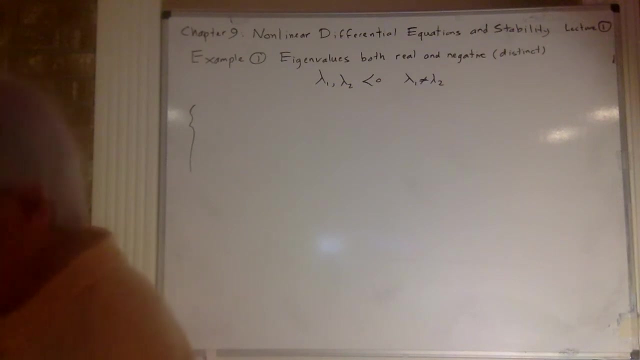 no, but i will tell you what this means. so let's uh start with this. so it is lambda one and lambda two. uh are not equal and they are both zero. they are only less than zero. okay, so example is this. let me copy, because then i don't want to just give you something. 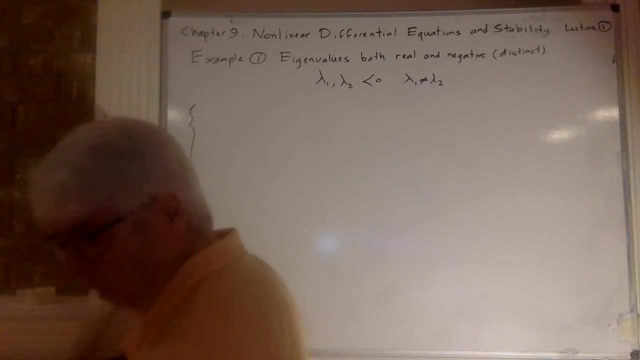 on the fly which might not have negative eigenvalues: minus three x plus four y. so x prime and minus three x and plus four y and y prime is: uh, i have x here minus three y. okay, so this is a linear system. a critical point is a zero, zero. how do you find it? just set them zero. 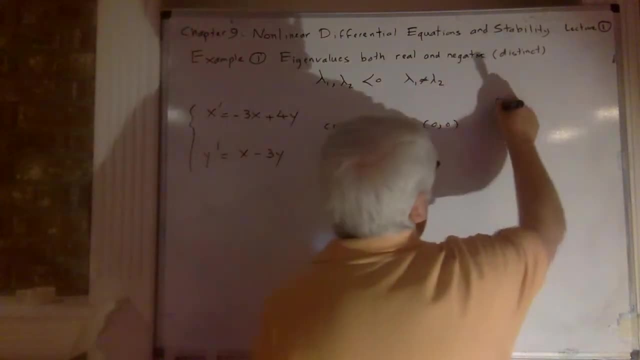 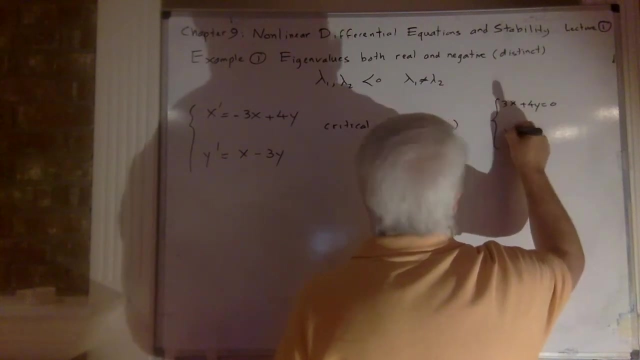 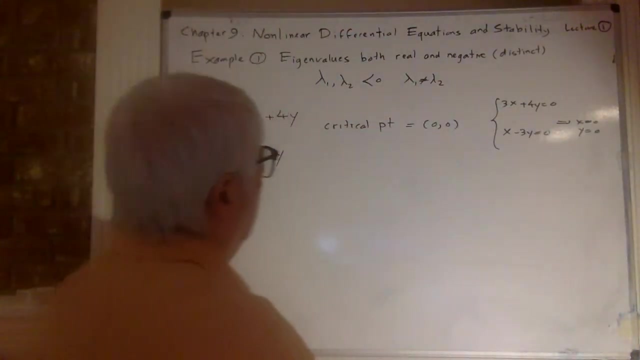 set this here. how do you find critical points? set this one and this one: zero. three x plus four y zero. x minus three, y, zero. that has only one answer. so critical point is zero, zero. at that point no slope is defined and the trajectory is zero, zero. 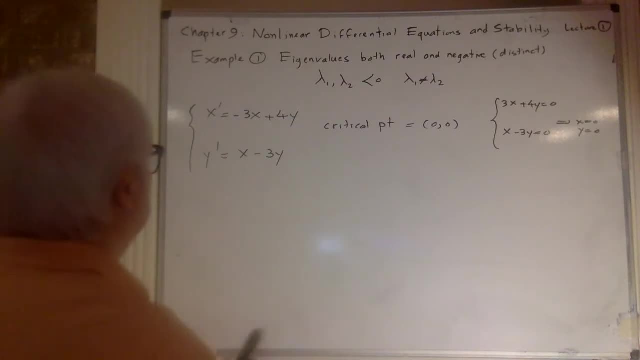 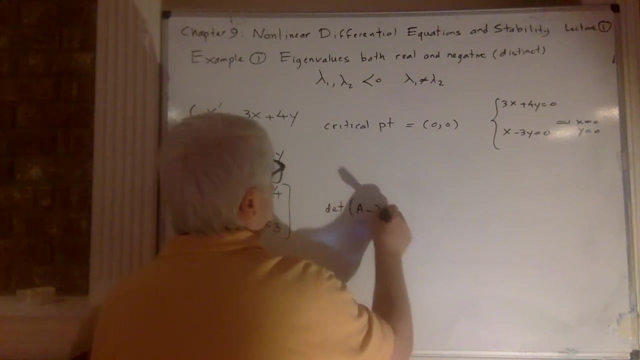 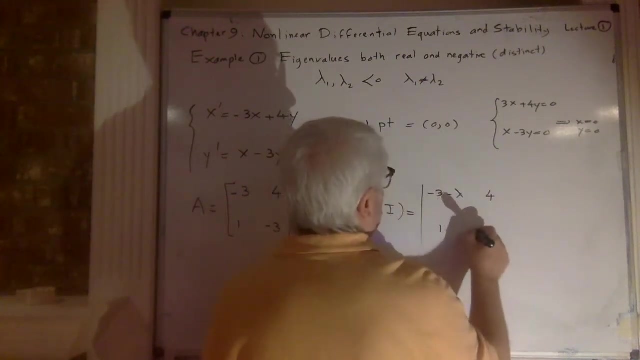 is never reached that point. no well, we know that we have the a, but what's the? a matrix of three, four and one negative three, so determinant of, say, a minus lambda, i is in fact minus three minus lambda. four, one minus three minus lambda, so that is minus three minus. 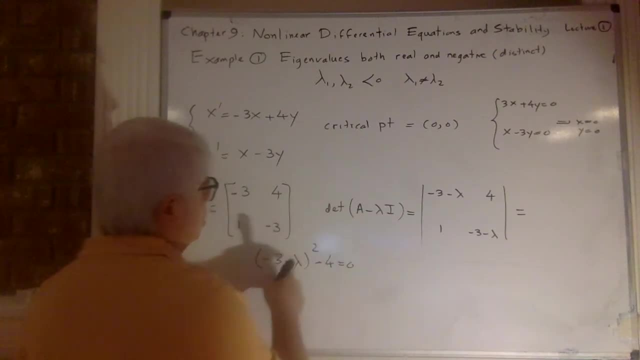 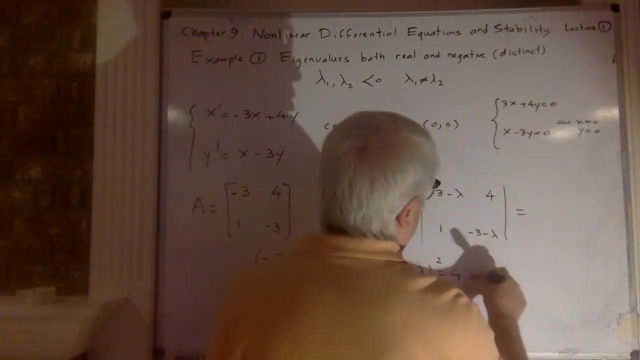 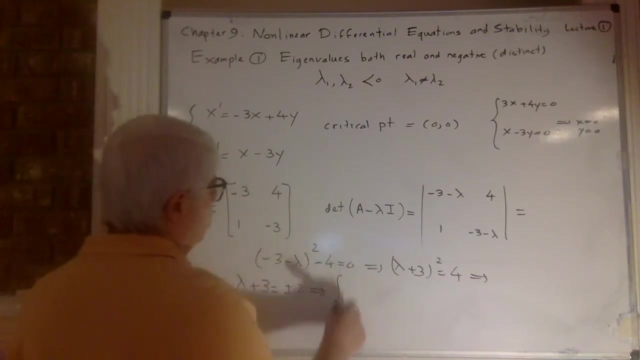 lambda squared and minus four is zero. this is the lambda plus three squared. so that is lambda plus three squared equals four. so lambda and plus three is plus minus two, and this gives me two lambda. then the one will be minus three. plus two is minus one. minus three minus two is minus five. 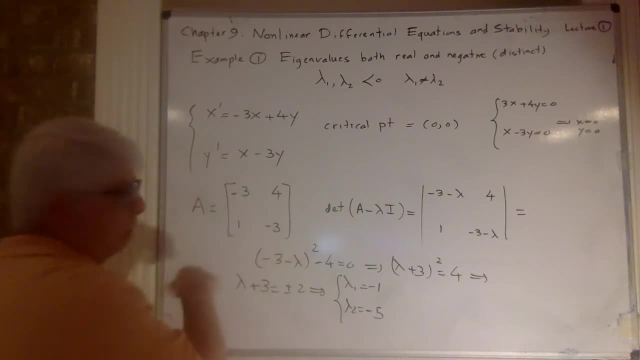 so whenever you have this, whenever these two are the same, then you will get something like this: that's lambda, plus or minus, something squared, uh. don't expand this thing because you can solve it like this easily. don't, because if you expand it will get the same answer. but you expand, then you have to use the quadratic. 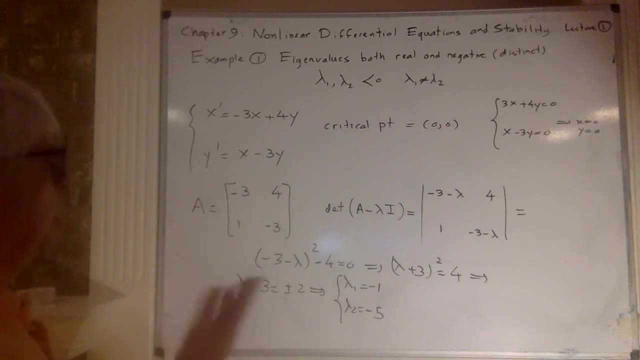 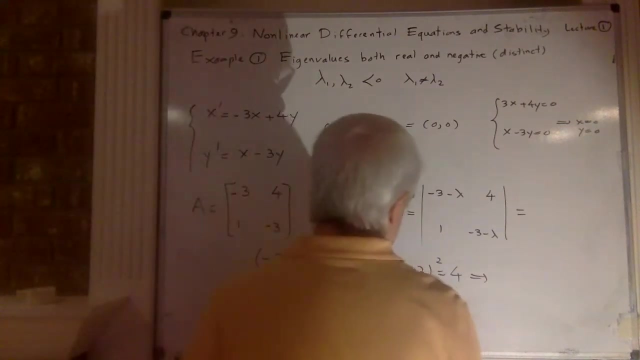 equation: uh, quadratic formula. but this is easy, so whenever these two are the same, just do this. okay, now i have found that i can get uh, there's no point in trying to find them, so v1 will be. this gives me the two eigenvectors: v1. 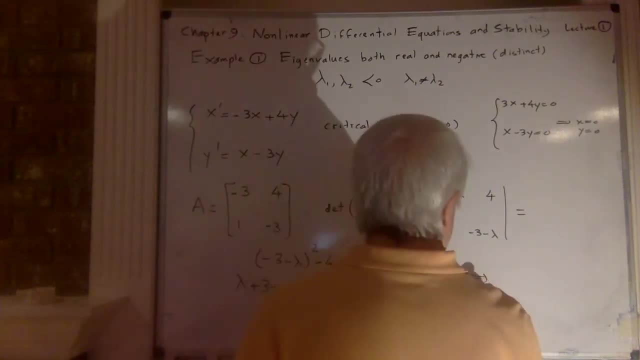 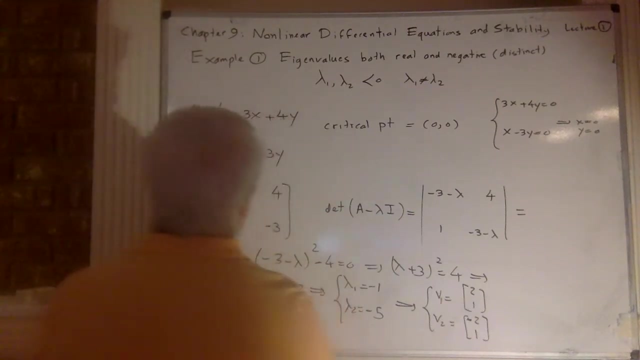 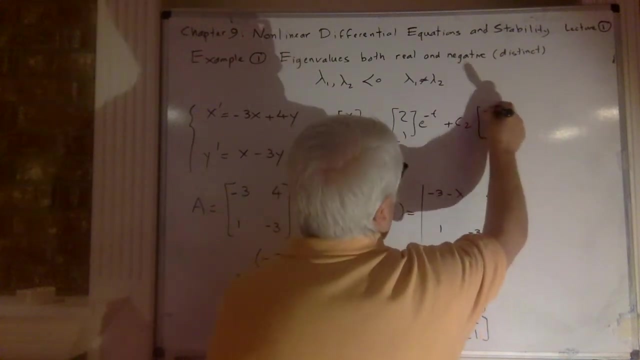 i found to be, it was the two one say, and the v2. i found v2 minus two, one. okay, so, so the solution, general solution, will be: uh, uh, the resolution will be this: x, y, c, one, two, one e to power minus t plus c, two minus two, one e to power minus five. 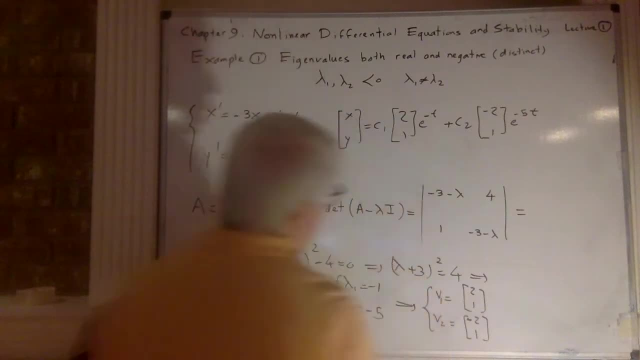 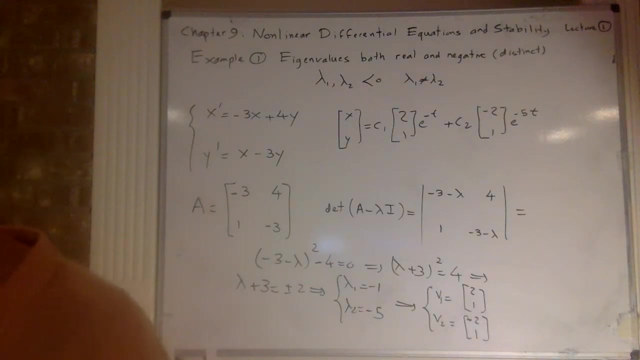 now i i have to give you i should start at some point in the face plane. so it's the. i have assumed the uh. it starts at point uh. let me see, let me check my notes, it starts at point minus two five. so let's assume that. 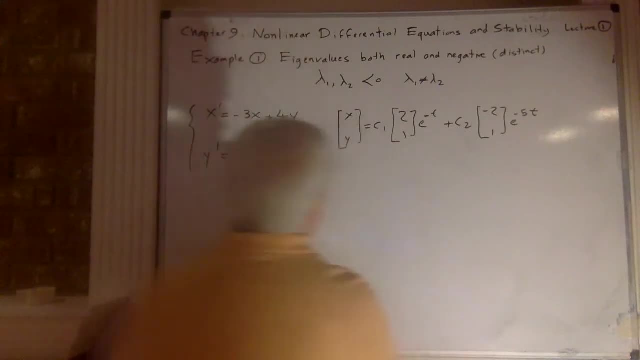 it starts at point minus two, five. so let's say x at zero is minus two and y at zero is five. so it starts at this point in the face play and uh, using sorry. so what is the list? this is in fact minus two is this is at zero. so it is two c one. 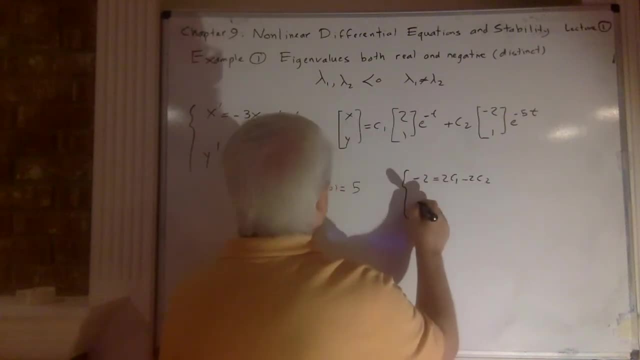 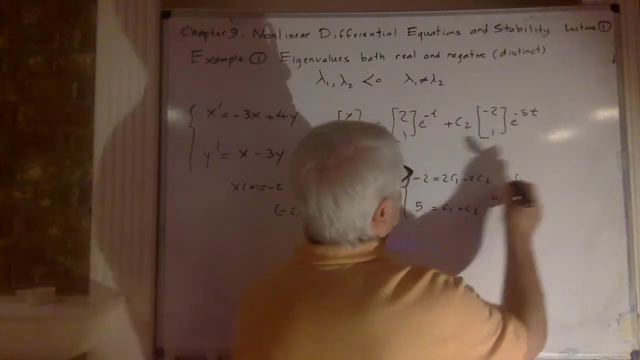 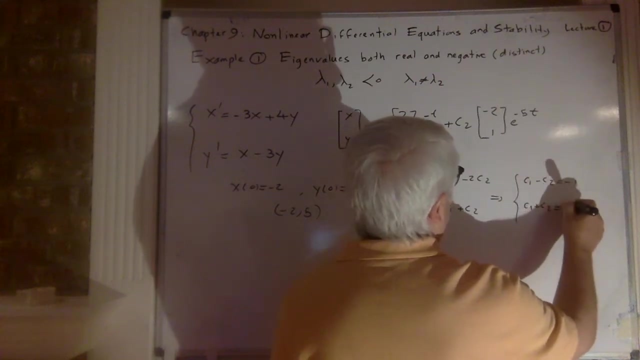 minus two c two, and this one is five equals c one plus c two. right, so i have c one minus c two is negative one, and c one plus c two is five. so if i add them i have two. c one is the four, so c one is two if i subtract. 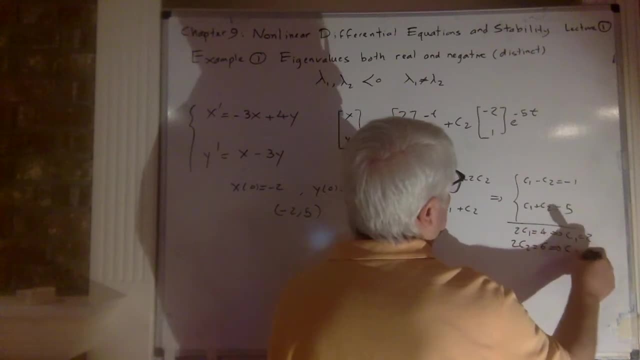 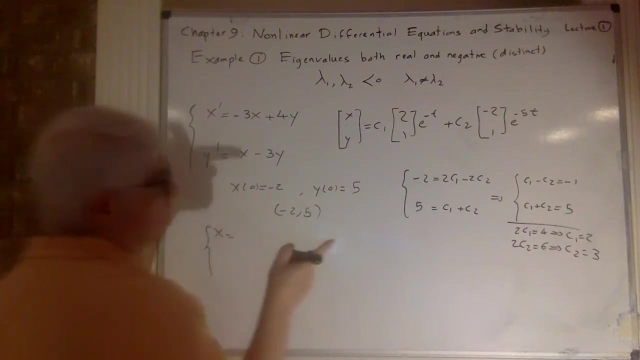 i will get two. c two is six, c two is three, so the solution is this: x is a, c one is two, so it is four e to power minus t and the c two is three minus six. e to power minus five t and the y will be c one. 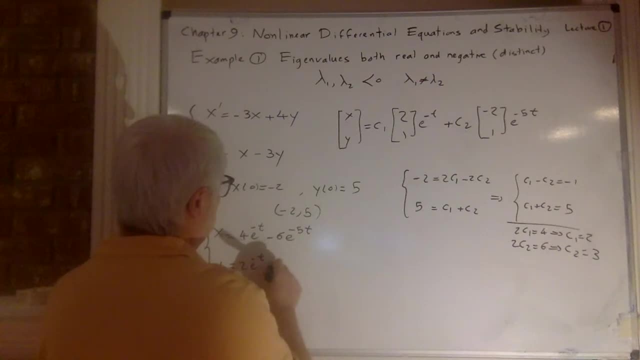 two e to power minus t and c. two plus three e to power minus one. okay, so i have said that and i say it again. so this is like parametric equations for the particle that is moving in a plane and it starts at this point, so at time. 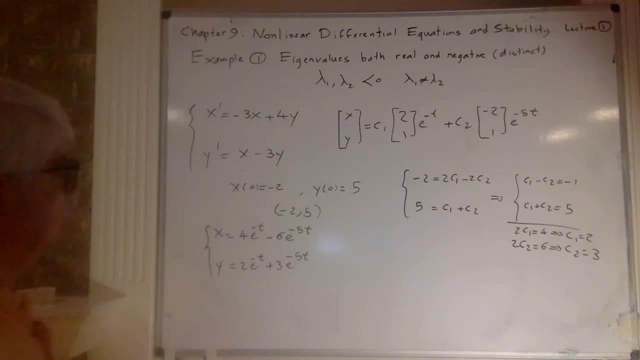 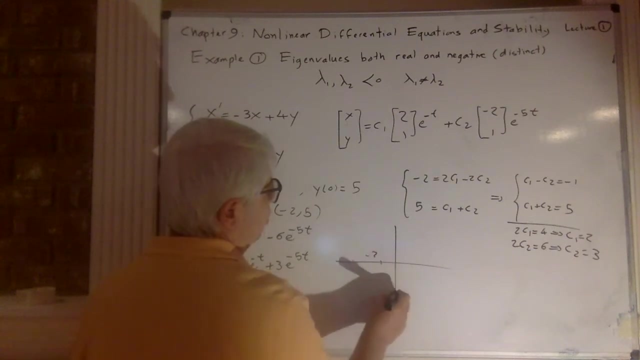 zero. it is at this point zero and i minus two and five. so so it starts here: minus two, say it's minus two, and five will be somewhere here. right, that's minus one, so five will be somewhere here. so it's somewhere like here, right? so at point minus two and five. 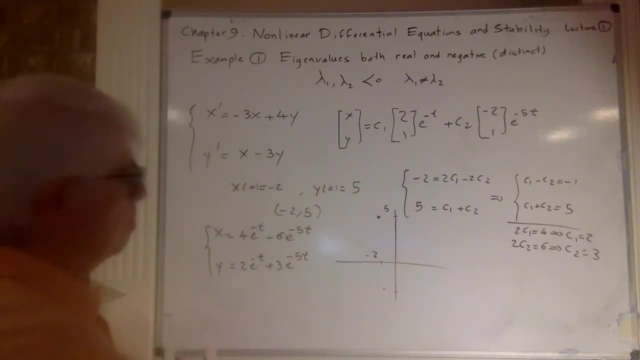 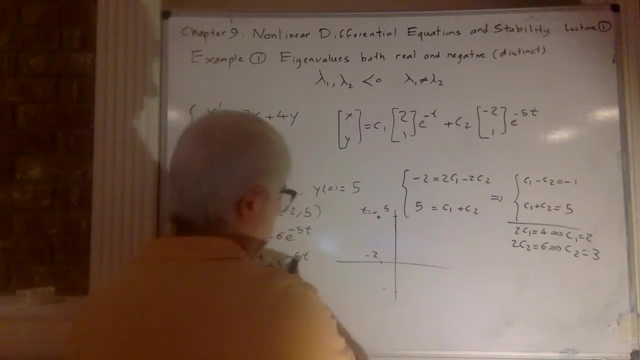 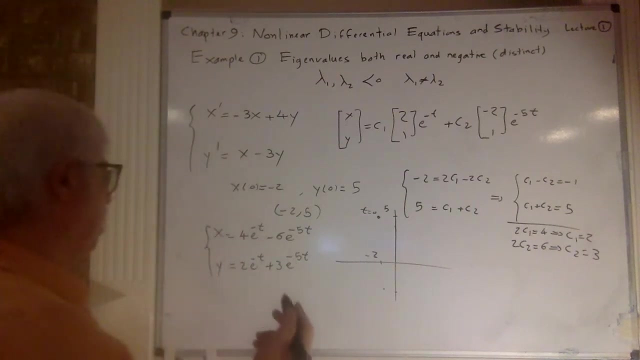 is this one say, and it starts as time passes. so this is time equal to zero. and if you graph this thing, if you parametrically plot this to uh, or just plot the, if you parametric, parametrically plot this on, say, mathematical, for example, parametric, 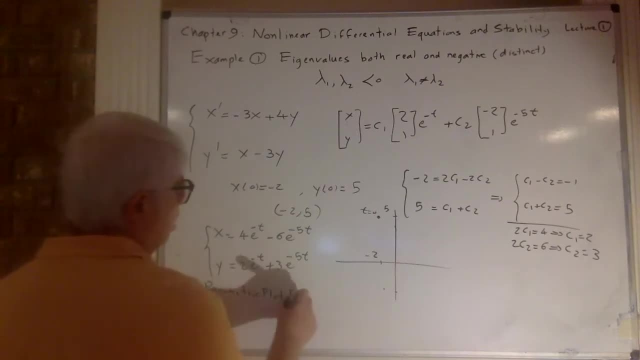 plot. if you parametric plot them: xt, xt and yt. let me just write xt and yt, or t from zero to say something: five, something, i don't know. uh, t from three to five, say then, uh, it will give you something like this: why i don't have a graphic? 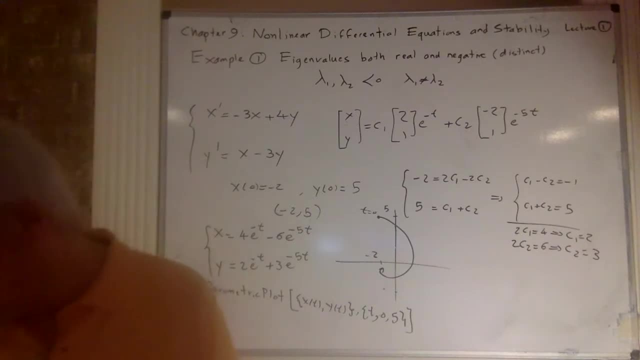 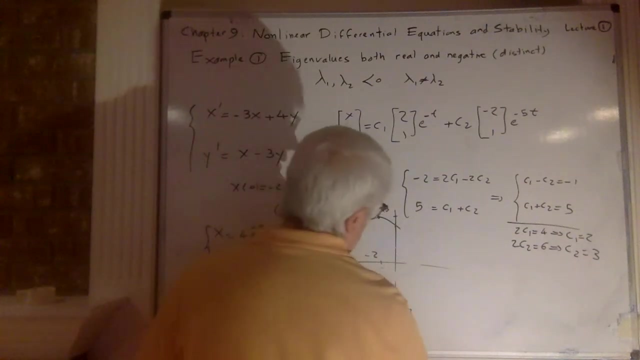 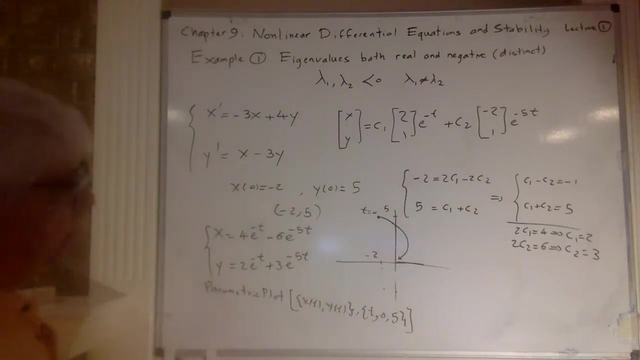 so, and i'm not sure it doesn't go, well, you know. so it goes back. yeah, it doesn't go below this thing. so it goes like this: it goes towards point zero, zero, okay, so torture, and gets closer and closer. it's interesting if you graph it for. 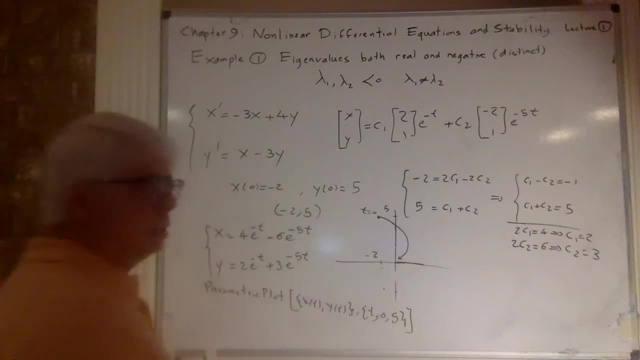 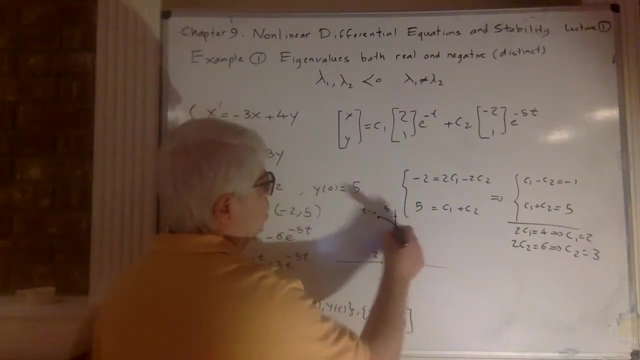 any time. just let the time be, say five, five million, it never reaches that zero, zero. it gets closer and closer and closer and closer. just imagine: uh, now one thing is, uh, why does it go this way? but let's, let's, let's look at this more. 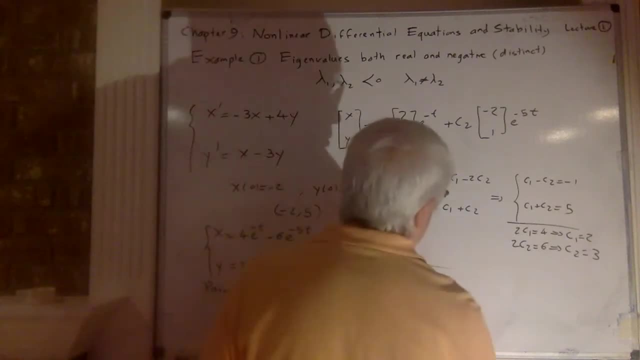 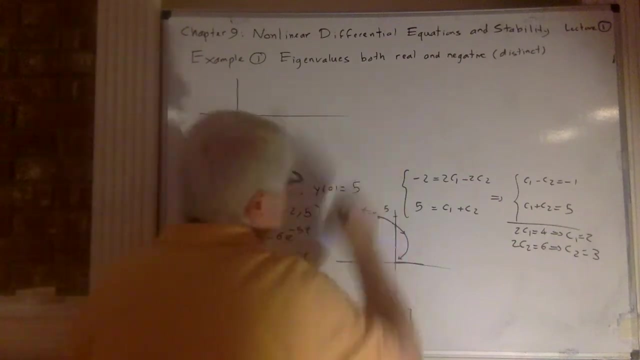 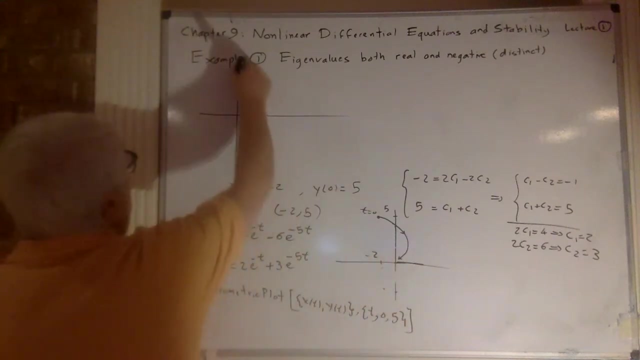 carefully. let me, uh, plot each one separately so you can see what they look like separately, and i have the two plots here. so that is, it starts at five and it goes like this: the other one starts at the negative two and so, okay, this, this guy here up here, is, 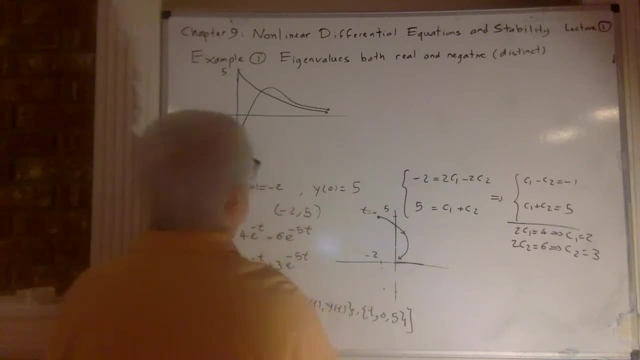 x. so let me so this up. here is the x of t, this guy, and this one here is y, and you can see that, because i assume that it starts at negative two. so you see, it starts on negative two. that's the x, and this one starts at five. it starts at: 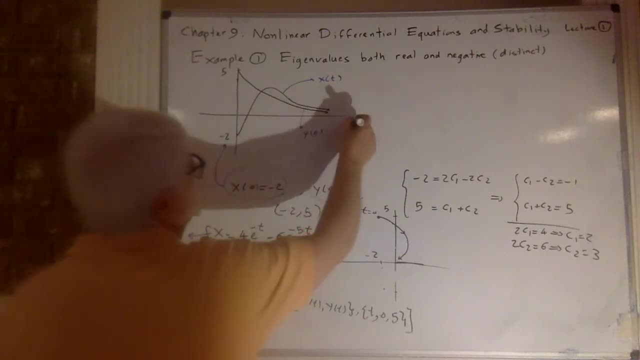 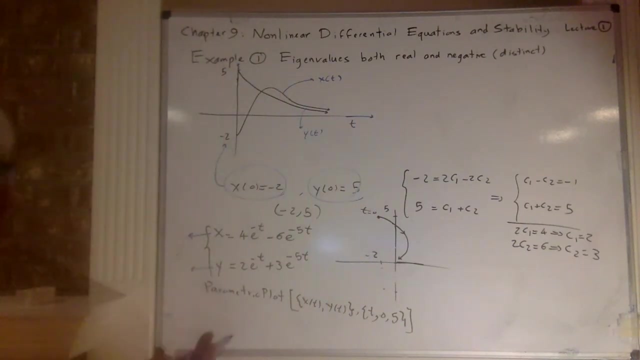 five. okay, and this is time, this is time, and this is the axis for both x and y. it's not x or y axis, it's just the the axis for these two. okay, so i i can. i have found some points, like to tell you what, uh, for example at: 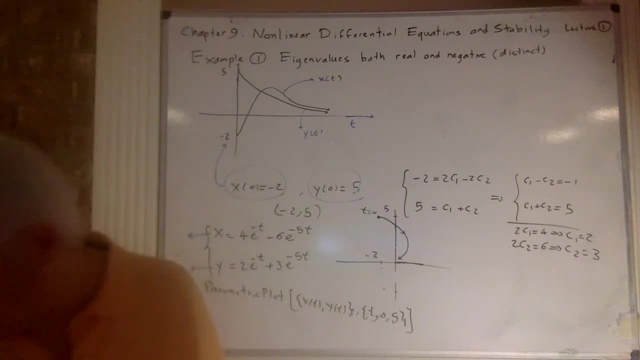 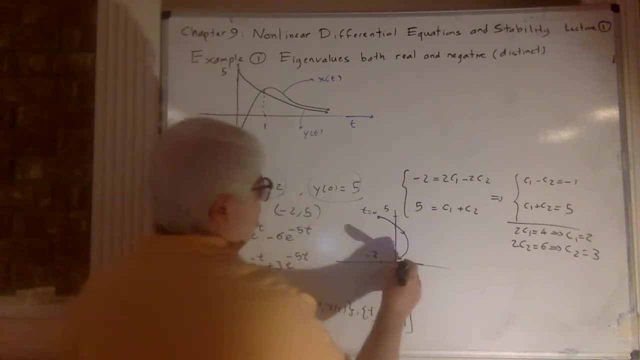 certain time say uh, certain time. so at time, because one, for example, a, it's almost, say so that time equals one. i calculated this. It's about: it's about 0.2 and 0.9.. So it is like: on this one it is like 2, is it 2?? So let's say it's 2 here and it's 0.9 here, Right? 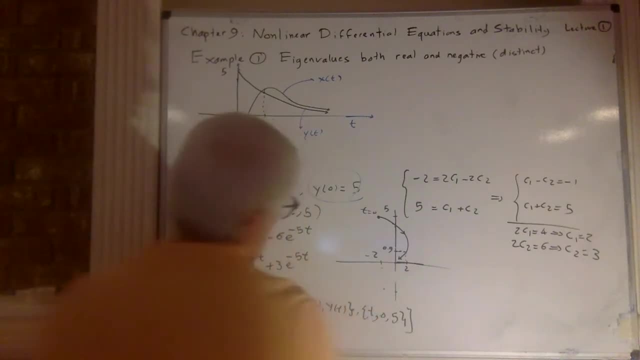 And what do these do on this picture? See, it can't be 0.9.. So this should be lower. That's going to be 0.9.. So it goes like this. Okay, So, for example, this one is 2, see. 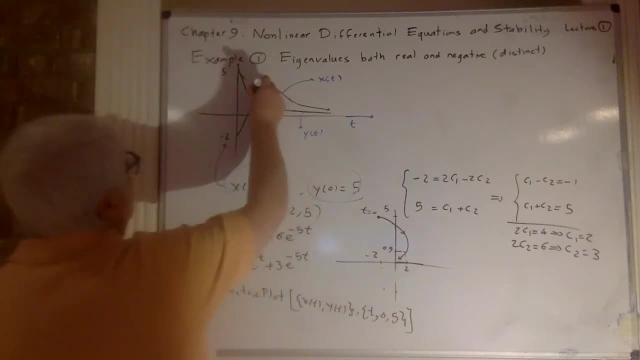 So that's the x and the y is 0.9, see, So this y is also 0.9.. Okay, So the 0.9 and 2.. And this is in fact this one, right? These two points give me this point. 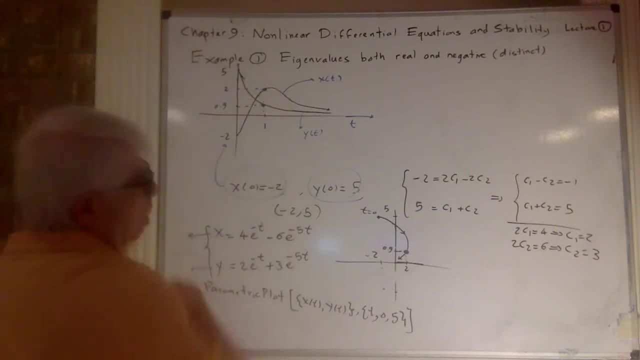 These two points, the x and the y, give me xy here. See, this is the x and this is the y, This x, that's y. So these are x and y separately. These two are x and y separately, And if I just take them for every time, this is time, So time is implicit here. You don't see time in this picture. 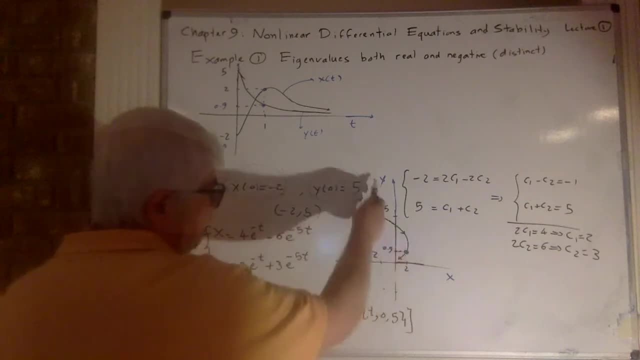 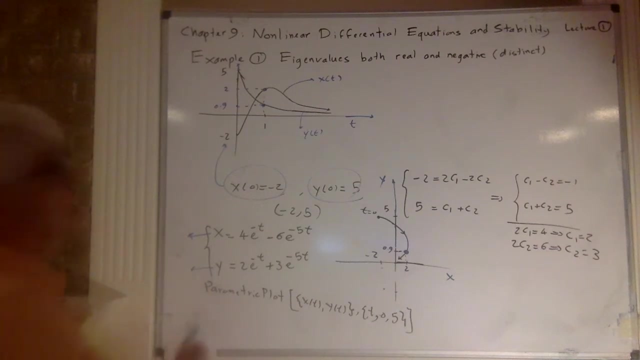 Time is implicit. Both x and y are functions of time. That's what parametric means. So time is implicit in this picture, In the trajectory, you don't see time. What you just see is that it is moving. So at say point, say 1 second, say it is like here: 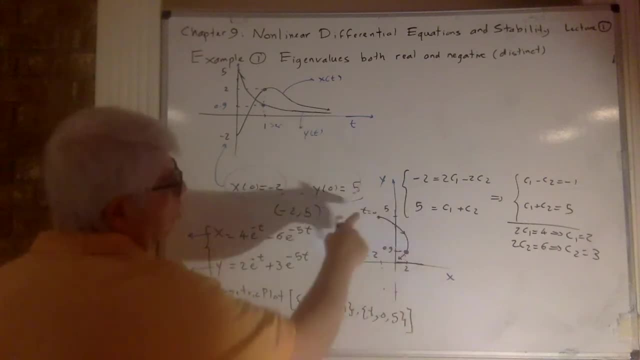 At point 0, it is 0,. 1 second, 1 minute, whatever that is, it is here And on this one you can see that the x is 2 and the y is 0.9.. I didn't calculate that exactly. You can calculate and find. 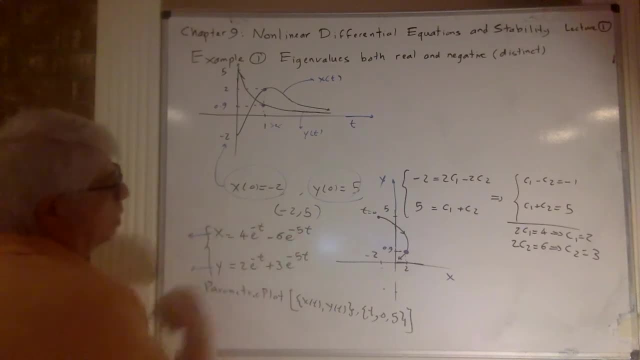 I'm not sure if for 1, you should put 1 here and find x and y Somewhere. Okay, So that trajectory is related to these two separately And you can see that this goes to 0.. This one also goes to 0. 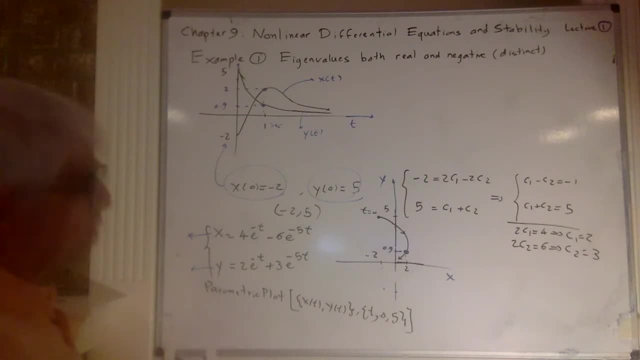 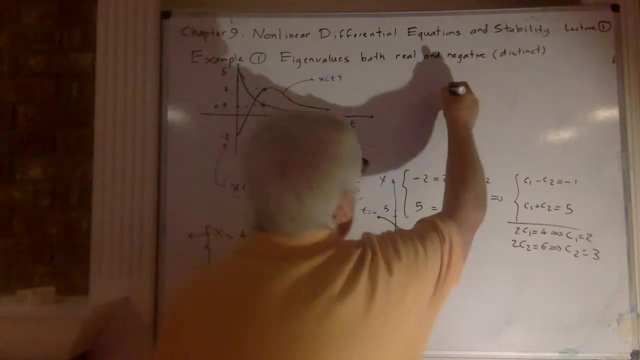 Why do they go to 0?? Why, when time gets larger and larger, they go to 0?? Look at these two. Look at x and y separately. X itself if you look at x separately. that is a linear combination of what. 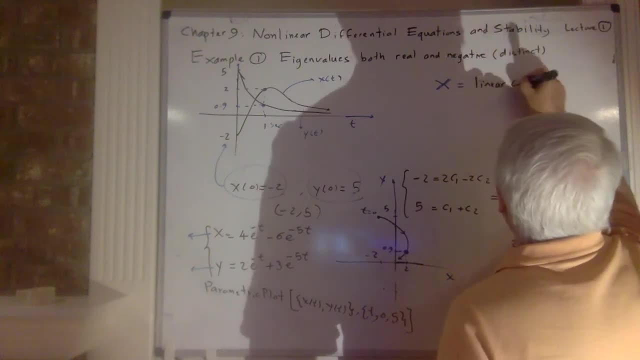 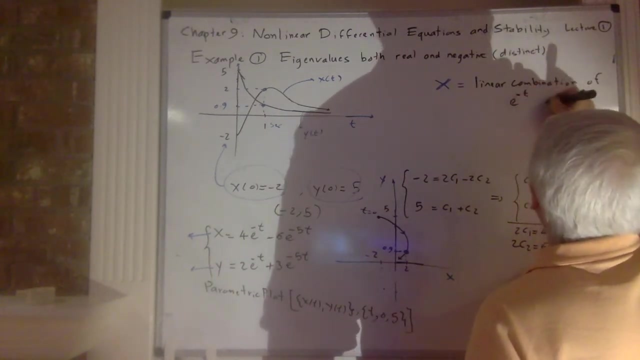 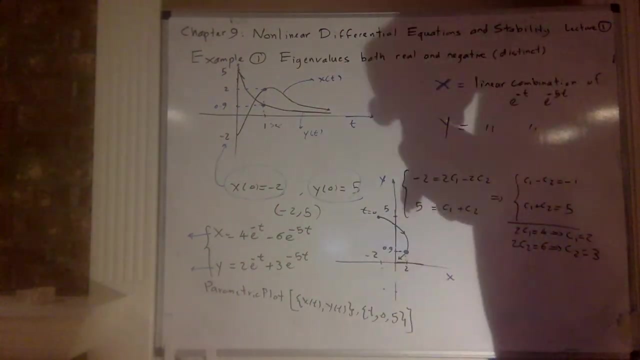 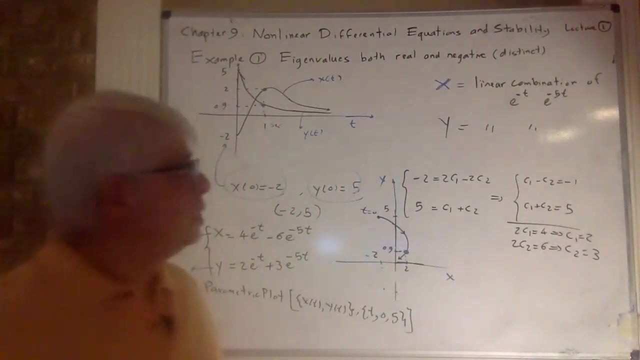 Linear, Linear combination of e to the power minus t and e to the power minus 5t. Why is the same? some linear combination. So each one of them is a linear combination of those two functions: e to the power minus t and e to the power minus 5t. 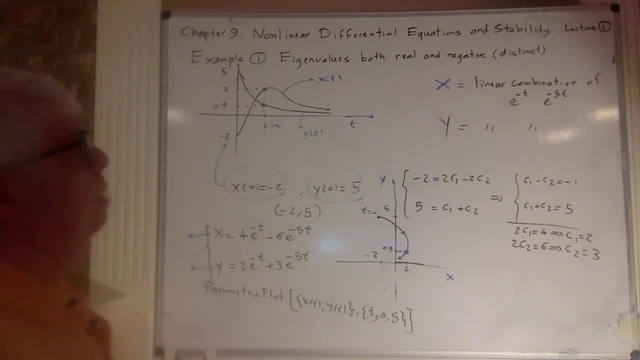 What do they look like? e to the power minus t and e to the power minus 5t. as t gets larger, That's minus t. So both of them go to 0, right? Each one of them is like this: 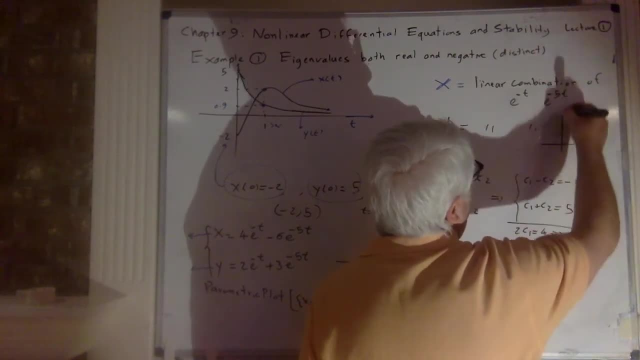 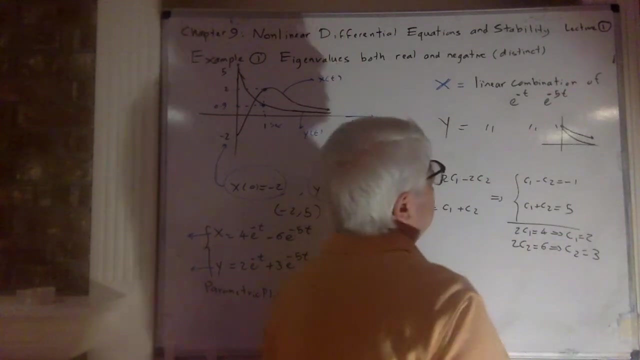 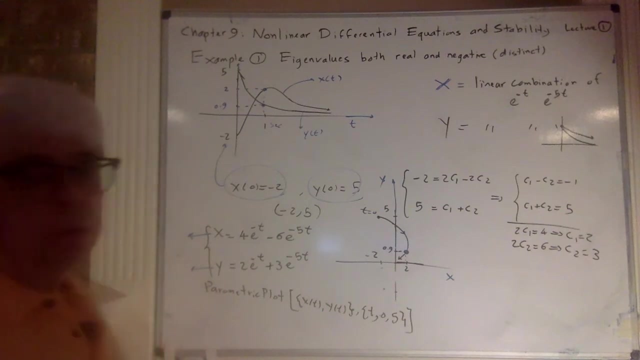 They start at t When t is 0, that's 1.. They start at 1.. e to the power minus 5t goes to 0, so fast, the other one slowly, So they both approach the x-axis. When they approach the x-axis, it means they are going to 0.. 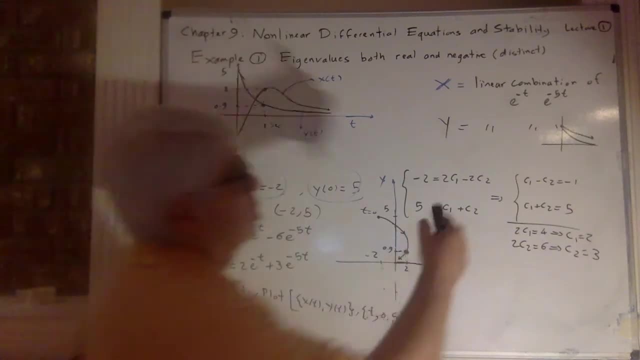 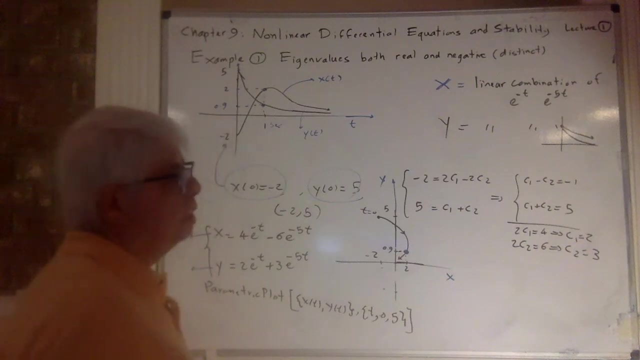 Because that x-axis shows just this. This is the value. So the value gets smaller and smaller and smaller, which means they are getting closer to the x-axis Anyway. so a linear combination of those two which becomes 0,, not exactly 0,, they approach 0.. 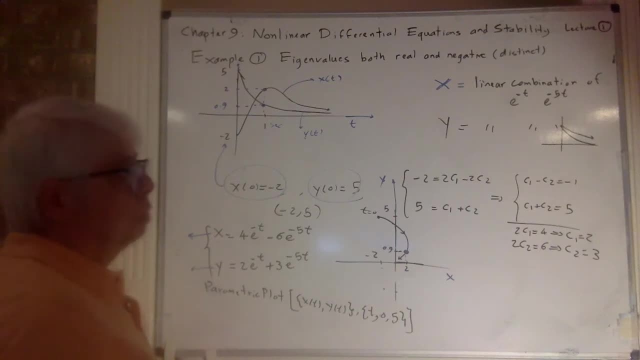 They are two very, very small numbers, Very small numbers, And the linear combination is just some constants times these two, So those constants really don't matter at infinity. At infinity, both of them are basically the same. They are 0.. 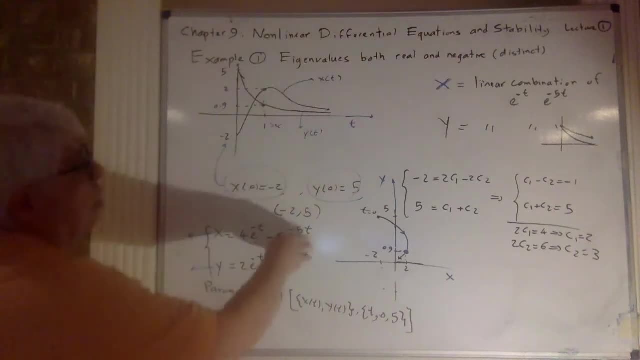 So this is like 0.000 something. The other one is 0.000 times 6 and times minus 6 and 4.. That will give you basically close to 0, not exactly 0. And you can see here, you can see that both of them are approaching the x-axis. 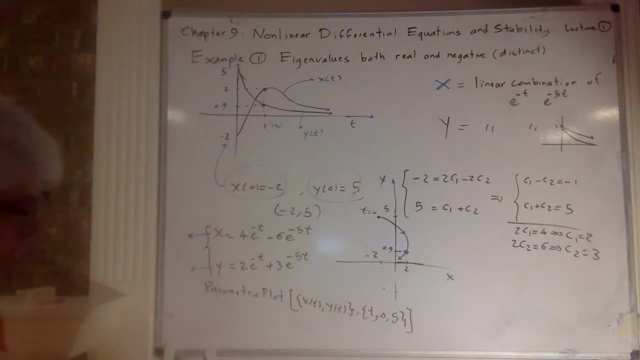 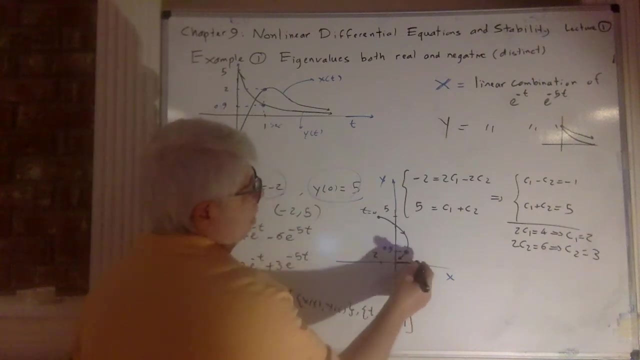 So the values are approaching 0. Now what happens here, Here, as they approach 0, this x approaches 0.. This y also approaches 0, right? So, as time goes to infinity x goes this way and y goes this way. 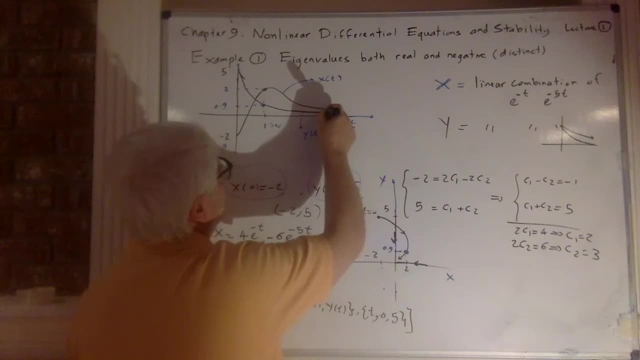 y goes this way, x goes this way, y goes this way. right, x this way, y this way. So here they are approaching the t-axis. Here, when you graph them together or put them together, this is approaching 0.00.. 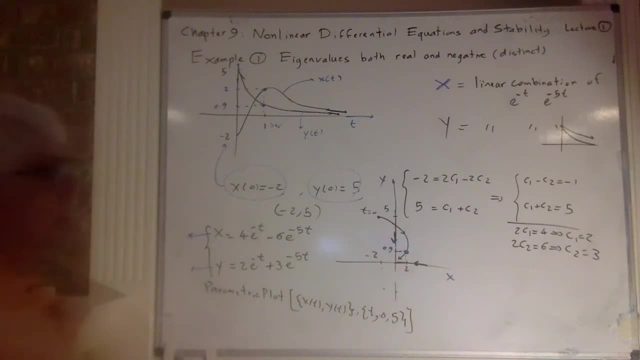 The trajectory is approaching 0.00.. Okay, So what do we say Just by looking at this thing, if that is the response of some system, So it's like I'm not saying it's vibration, it might be, but there's some system that it starts at time 0.00. 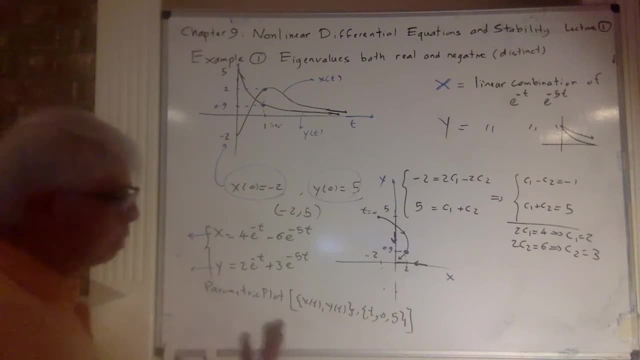 and the system, whatever the response is, whatever that is, it goes up, goes to 0.00. This one starts here and goes to 0.00.. So both systems- I mean both x and y, which are something related to a system- 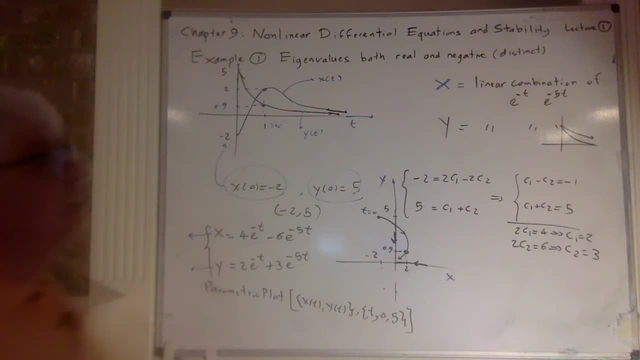 some values related to the system, some quantities of the system, like, for, if this system is a particle that is moving, for example, those are the x and y coordinates of the particle. So those two are going to 0.00.. And here in this picture, the face plane. 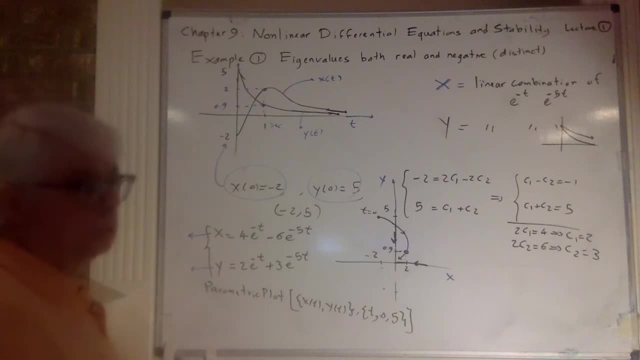 the trajectory is approaching 0.00, going towards the origin. We say that this is stable. As you can see, in the long run, physically speaking the system stops, But mathematically speaking it never stops, But physically speaking it stops right. 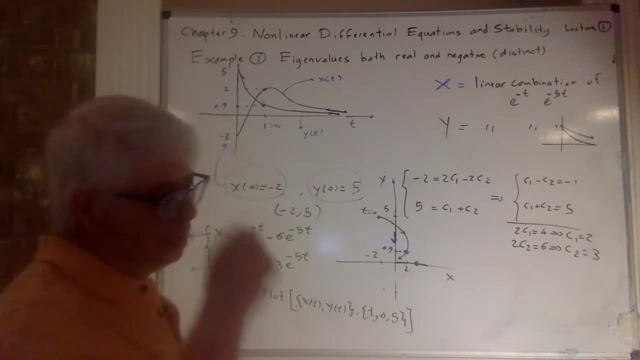 So in the long run you can say just: it's like vibrating very slowly, So in the long run it basically kind of stops. So that is stable. Now, why is it stable? As I had mentioned again, and I mentioned it again- 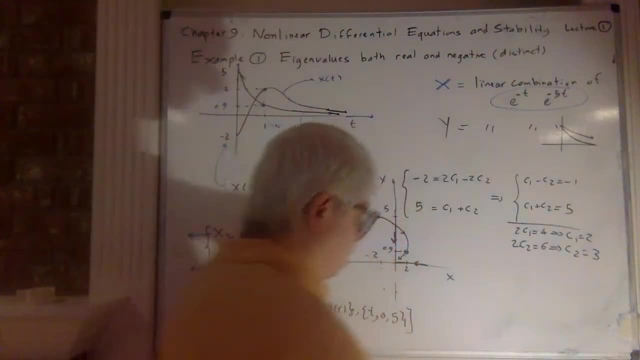 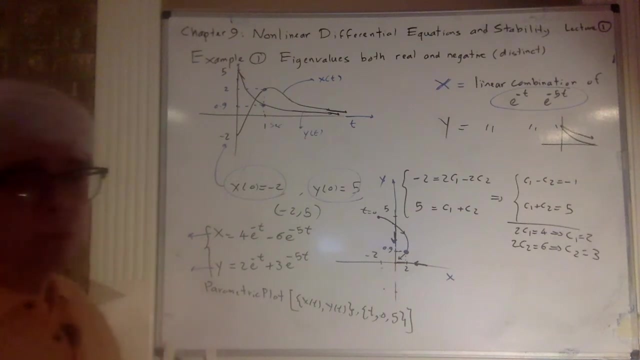 it's because of these two, Because of those two, e to the power of minus t, e to the power of minus 5t. they both become smaller and smaller and smaller and smaller. So any linear combination of those two, which any solution, is a linear combination of those two. 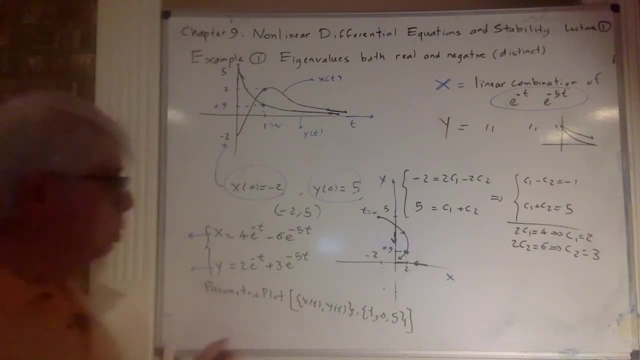 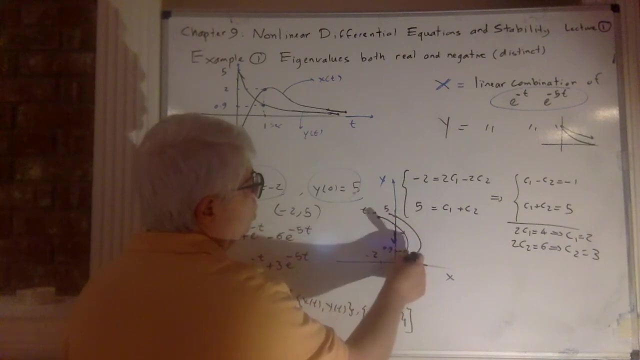 right, So that goes to 0.. Any solution goes to 0.. Any solution, which means if you start at any point it should go to 0.. OK, Any point. So if you start, say here, it should go to 0.. 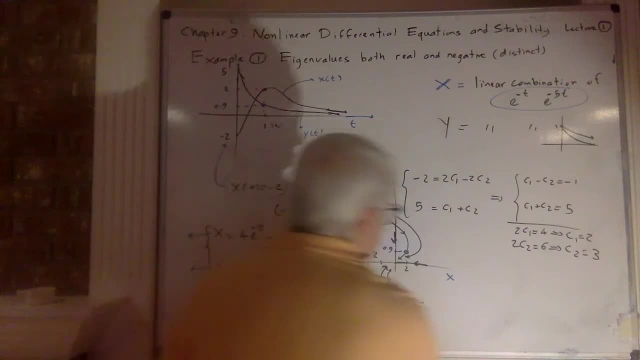 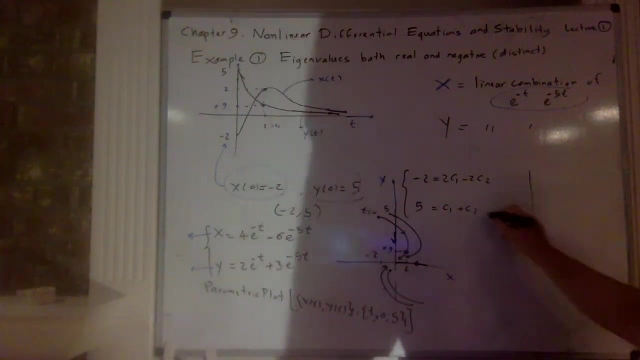 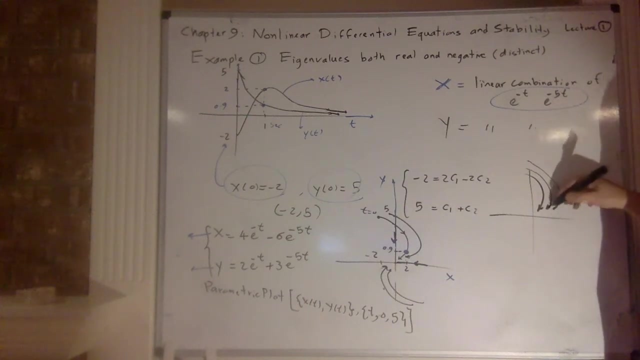 And, in fact, the face plane. if you graph the trajectories in face plane on a ball from opera, for example, or mathematical, if you have it, you will see that they are like this: They don't intersect, In fact, they never intersect, but they get closer. 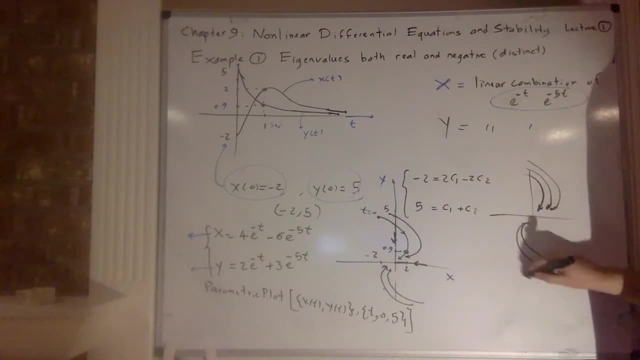 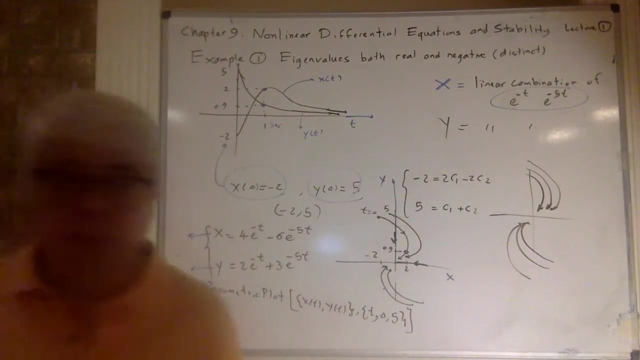 closer to 0, this way, This way, OK. So all the trajectories go towards 0.. Wherever they start, wherever they start, wherever they are at time, 0, they might be way up there in the universe, somewhere in the universe. 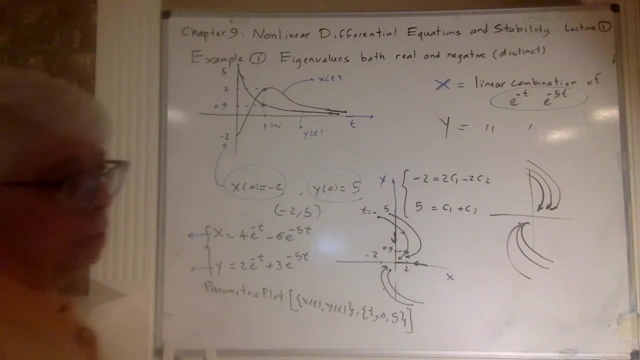 Eventually, if that 0, 0 is like the earth, for example, they get closer and closer to the earth. OK, So that is the story, when- No, Well, I didn't finish the story. So these two are related to this: minus t and minus 5t, right. 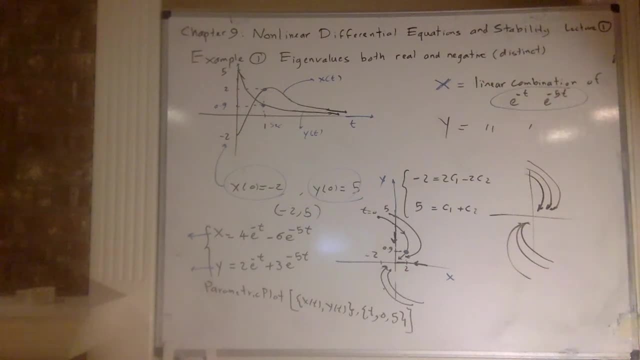 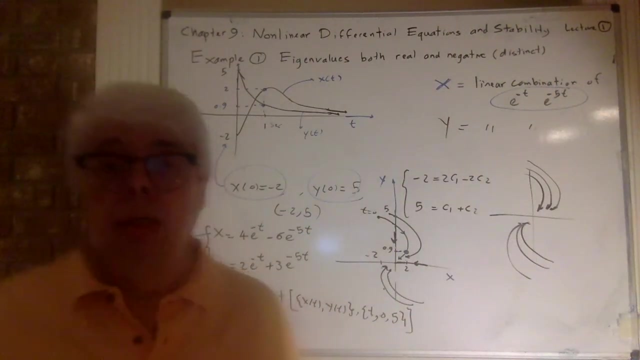 So where do they come from? That is minus 1t and minus 5t. Those were the eigenvalues of that system. right, Because the eigenvalues were negative, these are better. So two negative eigenvalues give me stable solutions. 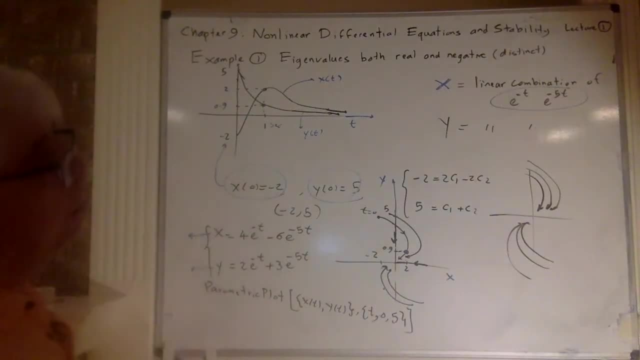 All of them are stable Because all of them have that e to the power minus 4t and e to the power minus 5t. So we can conclude, if we have, So, because in general, if the two eigenvalues are negative, 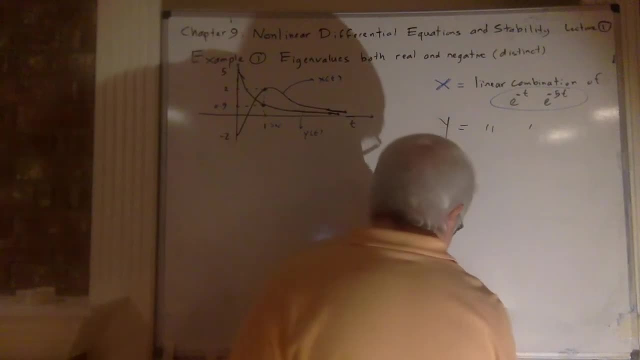 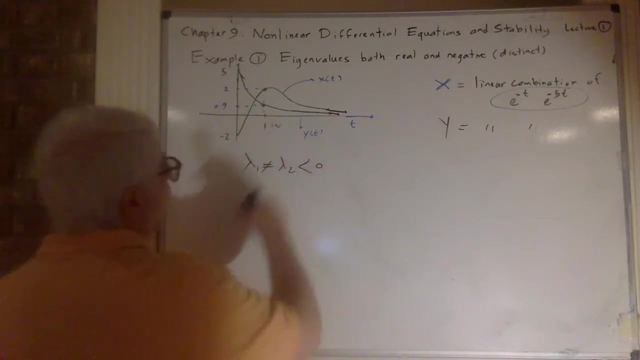 Yeah, I have written here- I didn't erase that. So if the eigenvalues are negative, y1 is not equal to y2 and both are negative. then I have e to the power lambda 1t and e to the power lambda 2t. 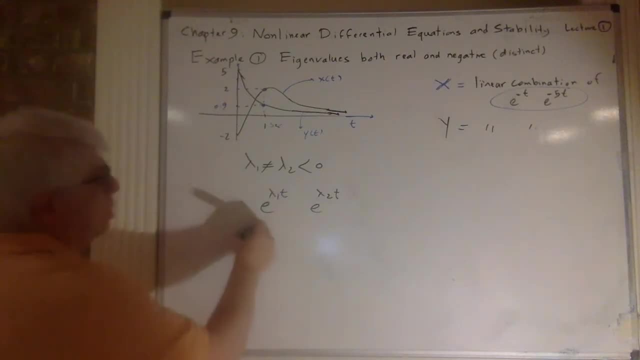 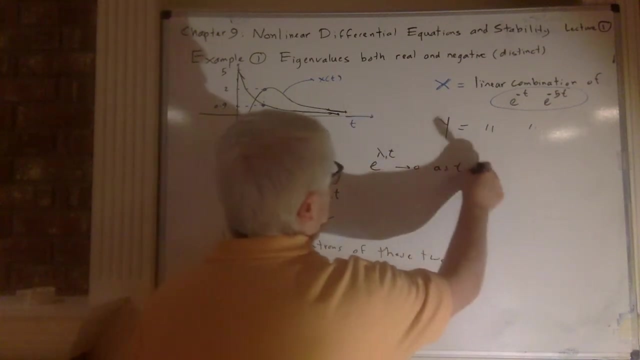 And solutions are linear combinations of these two, right, Linear combinations of these two, And I know that if they are negative, both of them are like this: They both go to 0 as t goes to infinity. lambda 2t also goes to 0 as t goes to infinity. 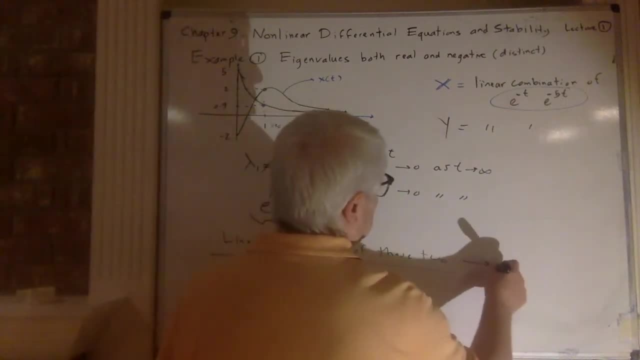 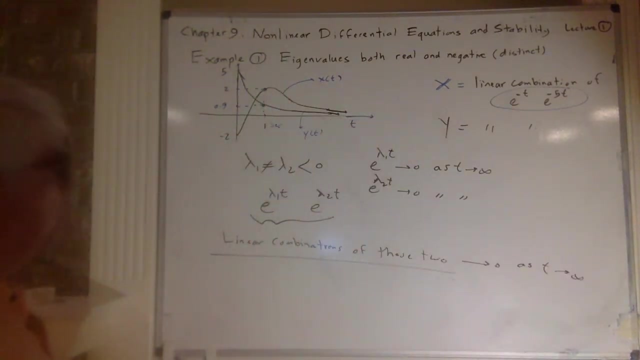 So any linear combination also goes to 0, as t goes to infinity. So we call this situation- because they are all getting close to 0.00, we call this thing a stable node. So a stable node is when lambda 1 and lambda 2 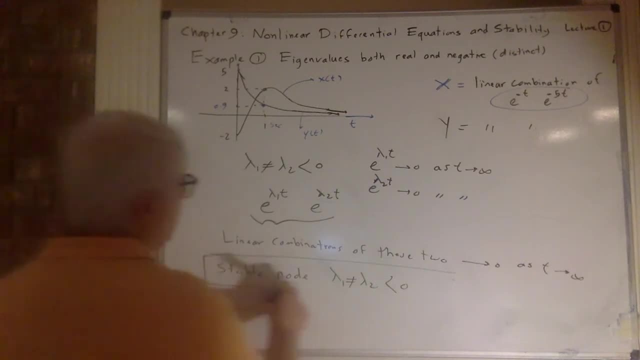 are distinct and less than 0.. Okay, So that 0.00 is called node and lambda 1 and lambda 2 are distinct and less than 0. So this is the situation that we have stability. Now what happens if they are positive? 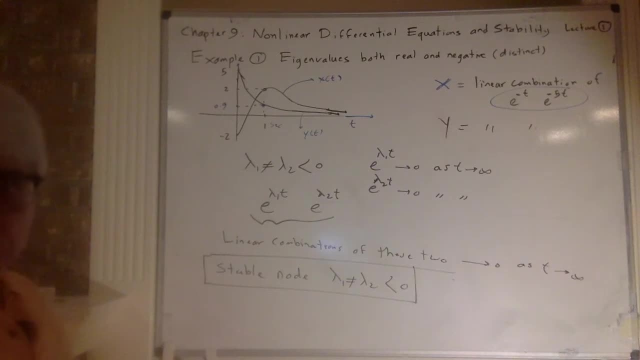 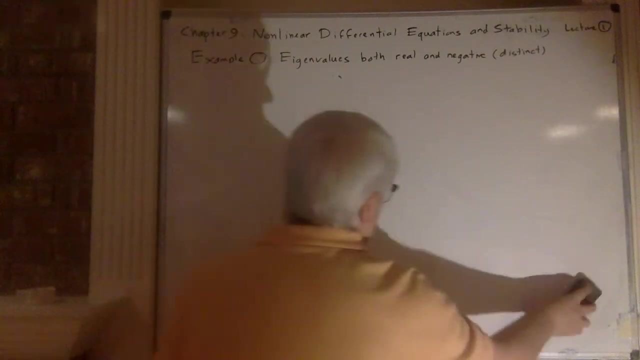 Well, you can guess. Positive means what They go the other way: Diversion. Well, let me write another example for you. Let's Example 2.. Let me write this down. I've written here, And In fact this should be written asymptotically: 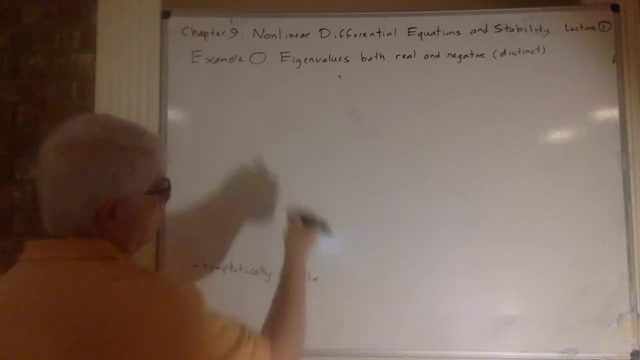 Stable And you know why. asymptotic means that x-axis or the t-axis is the asymptotic Right. Because the t-axis is the asymptotic, It's horizontal asymptotic And the point is: 0.00 is like. They approach that asymptotically. 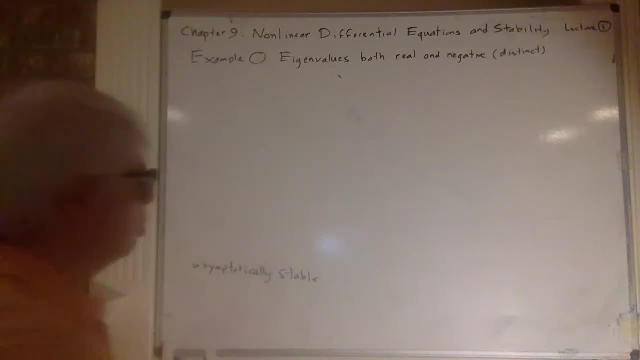 They are approaching this asymptotically: a stable node. So really, that's the only situation When the eigenvalues are both negative and distinct. Okay, So example 2, again I wrote an example which, In fact, that's the opposite of this. 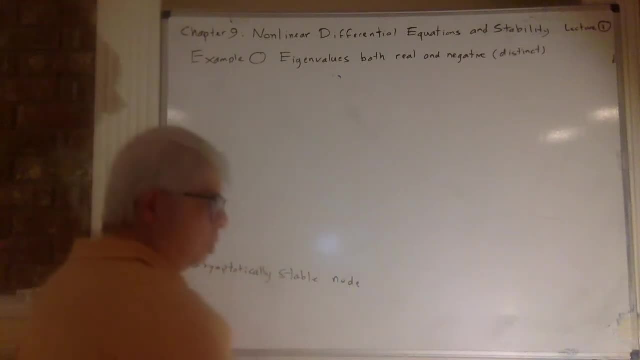 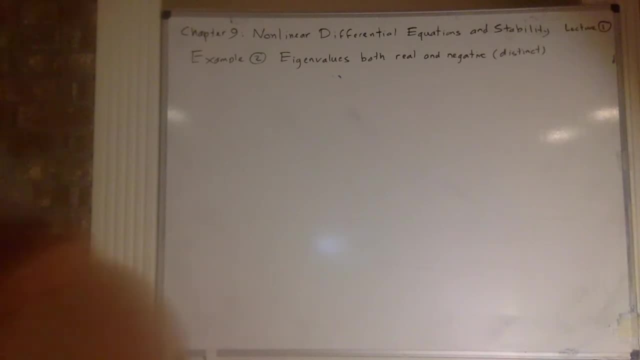 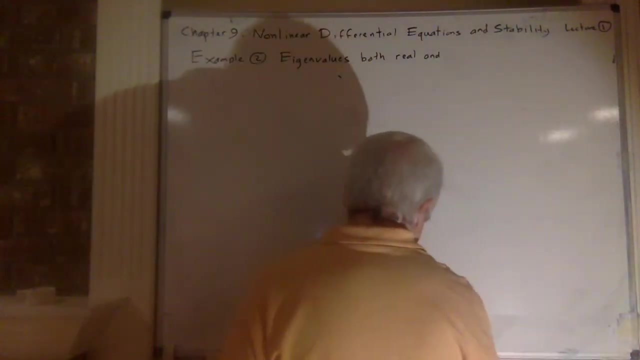 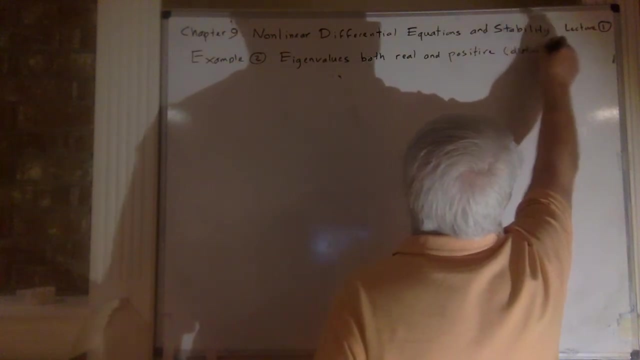 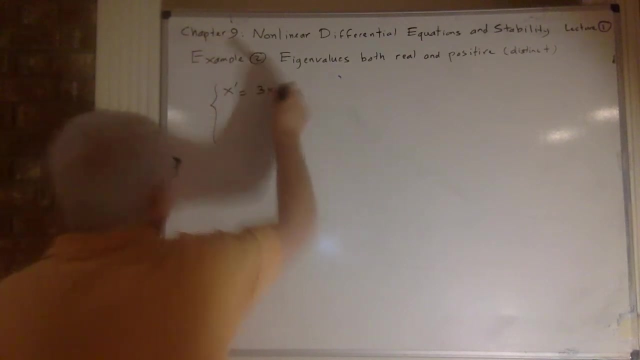 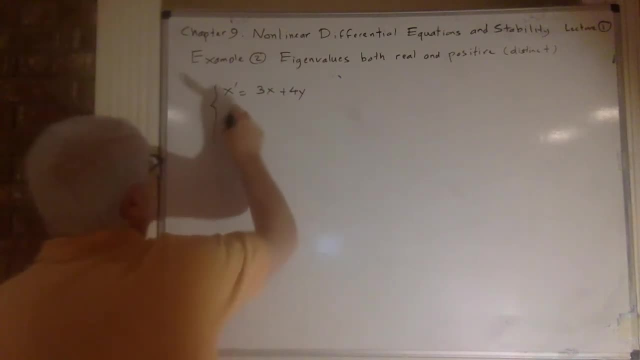 So. So y' is x plus 3y, so the A matrix, the cohesion matrix, is 3, 4, 1, 3. again, you see these two are equal, so this one is easy to solve. only the quadratic formula. so the determinant of 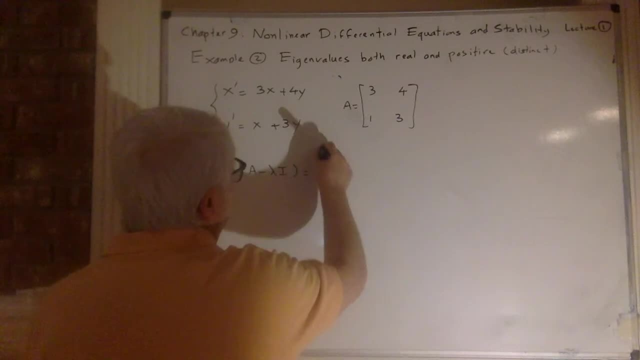 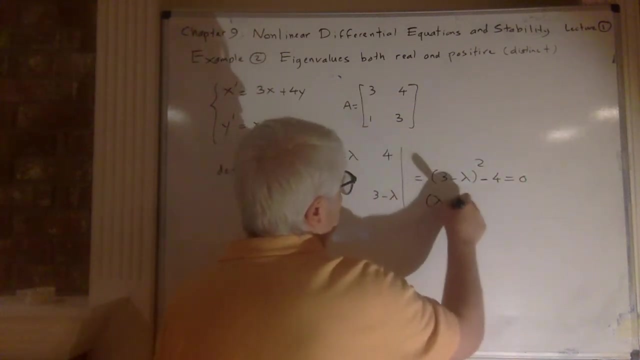 A minus lambda R is 3 minus lambda, 4, 1, 3 minus lambda, so I have 3 minus lambda, squared minus 4, again equal to 0. I can write this: lambda minus 3, no difference, right, just multiply by negative 1 inside and nothing happens. equals 4, so lambda minus 3 is plus minus 2, so lambda. equals 4.. So lambda minus 3 is plus minus 2, because lambda 2 is 2 and lambda 3 is 3 and lambda minus 3 is plus minus 2. so lambda minus 3 is plus minus 2 and lambda minus 3 is plus. 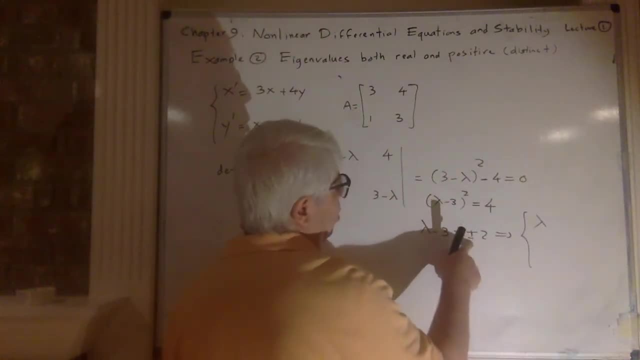 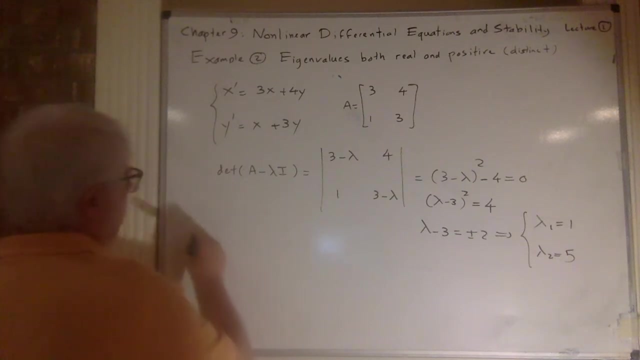 is 3 minus 2 is 1 and 3 plus 2 is 5. well, you can see that I got the two answers, but the opposite one, so 1 and 5 and v1. that gives me v1. I can't remember v1, I guess because of the opposite of those two, v1 is minus 2. 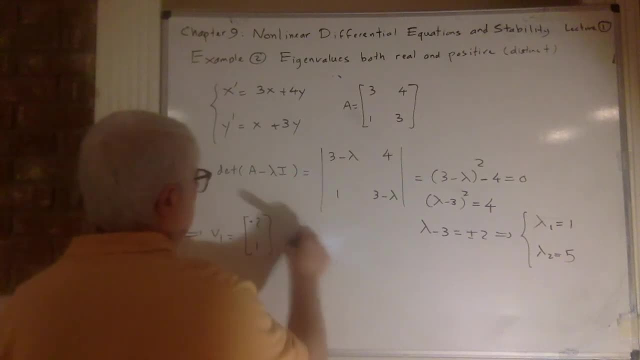 so the two solutions will be like this: there is everything, and the two solutions will be x and y, c1 minus 2 and 1 minus 2 and 1 plus c2 and 2 and 1. now I start this. one at minus 2 and minus 3. 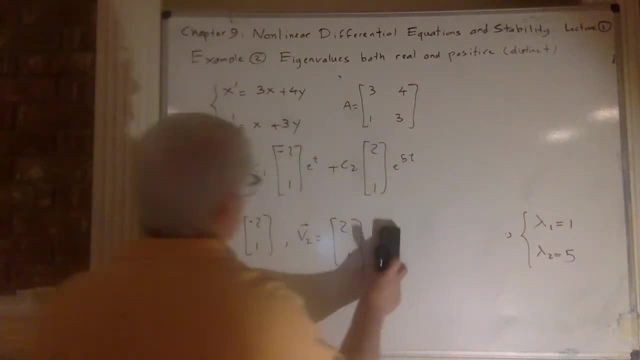 so let's start at minus 2 minus 3. so let's say x at 0 is minus 2 and y at 0 is minus 3. so just do the same thing and I think that's it. so let's say x at 0 is minus 2 and y at 0 is minus 3. 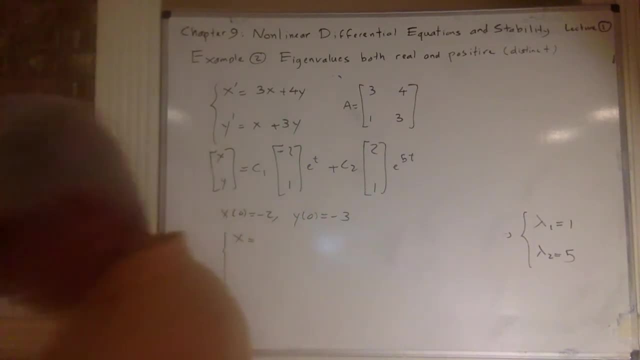 so I found x to be: x is 2 e to the power of t and it's 4 e to the power of 5 t, and y is minus e to the power of t and it's 2 e to the power of 5 t. 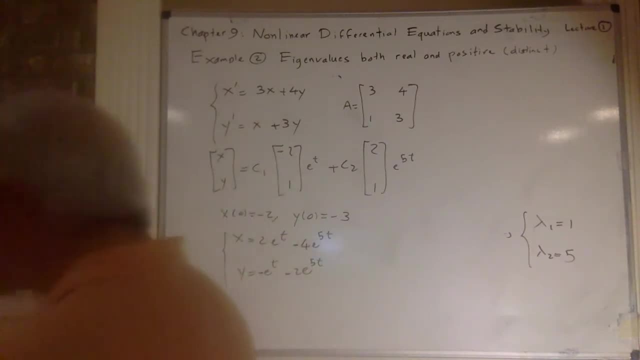 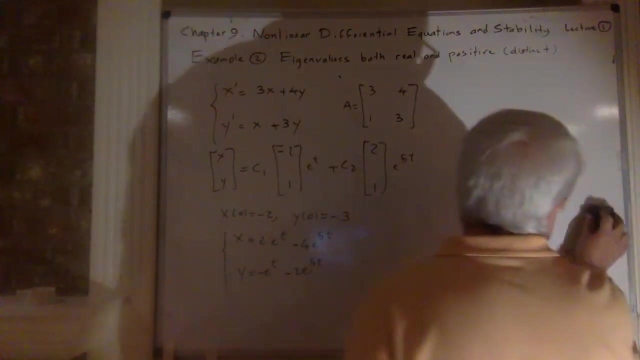 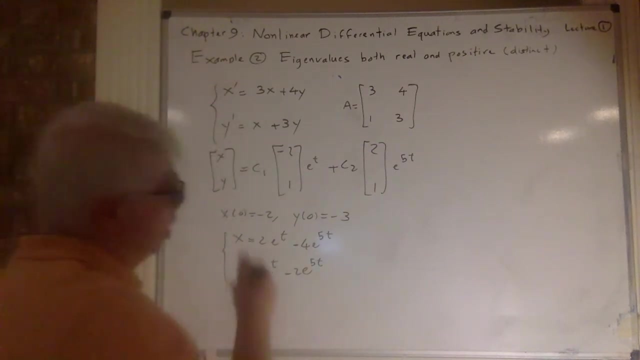 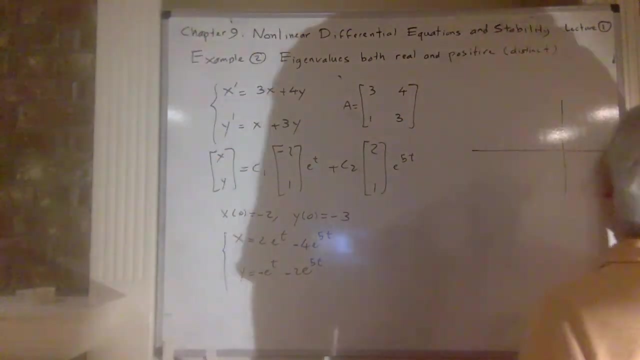 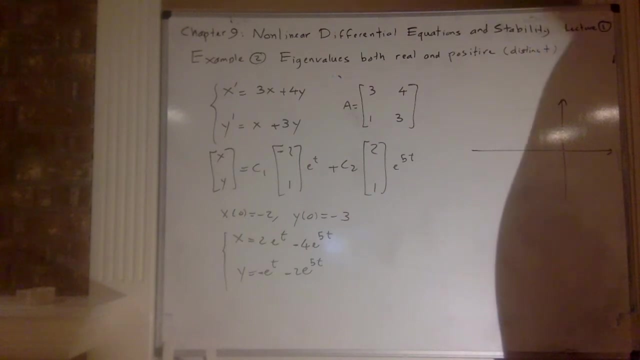 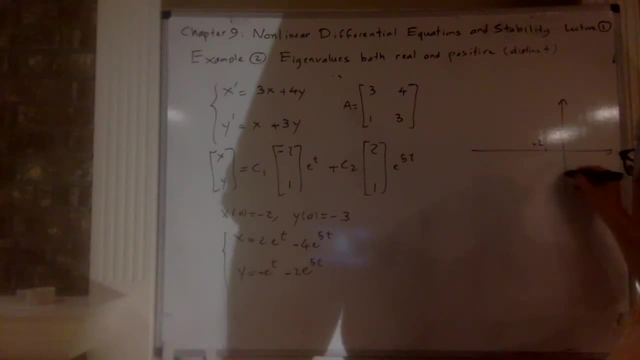 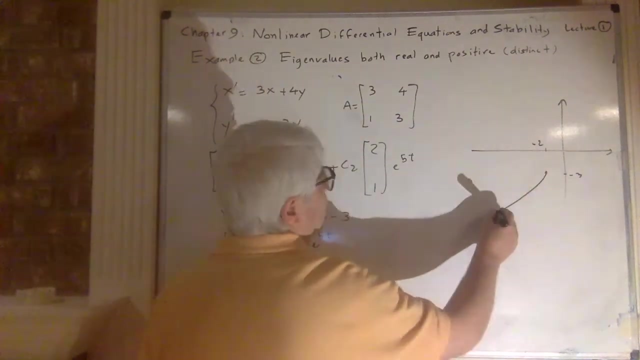 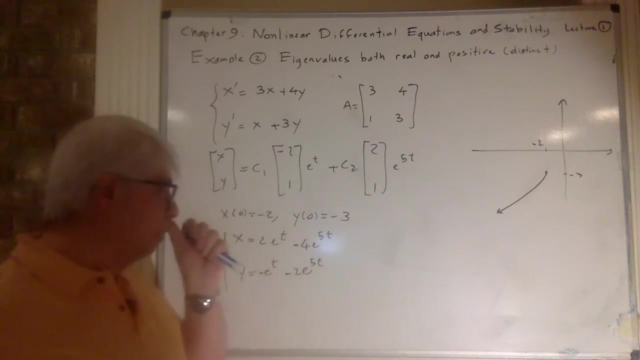 so if this is negative 2, say negative 3, it starts somewhere here, right, and then it just escapes going this way. and you can see why it goes this way: because this e to the power minus 5t, as t gets larger and larger. this is larger than this. 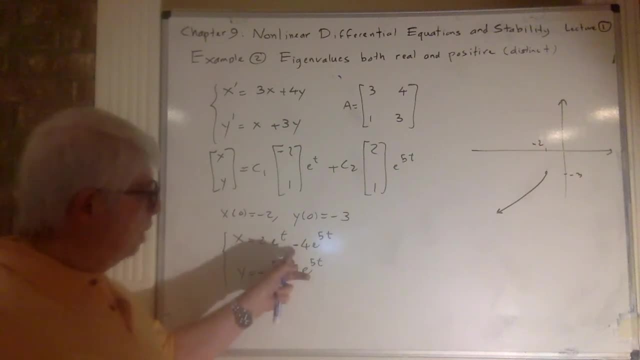 and both are negative. this is minus 4 times. this is minus 2 times this. so this, these two dominate this. e to the power 5t. when t is say 5, 10, for example, that's e to the power 50. this is e to the power 10. this is way bigger than this. so this is too negative, it just 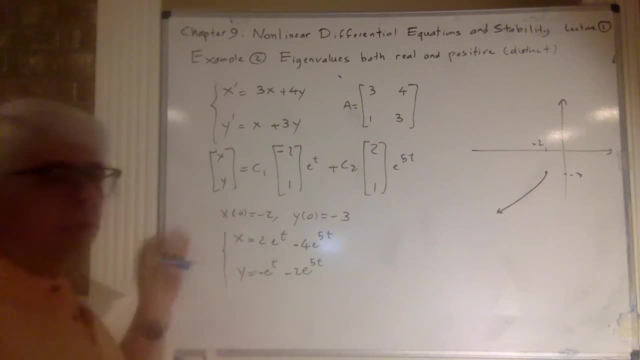 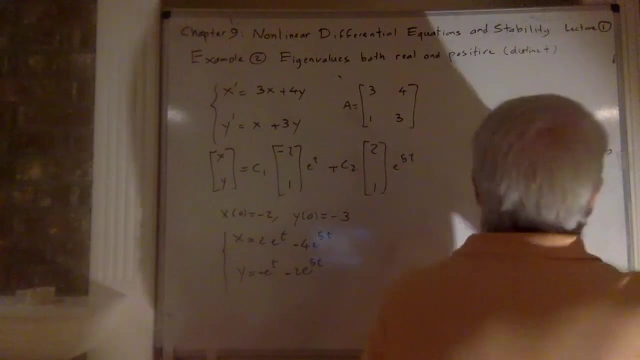 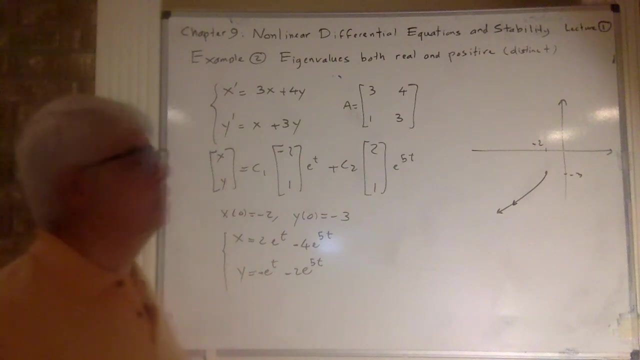 eats this one, say it dominates the other one. so that's why you see that it goes to infinity this way, both negative and well you can guess that this. well, it starts at time zero. what if you assume that there is negative time? you can see that it gets closer to zero in negative time. 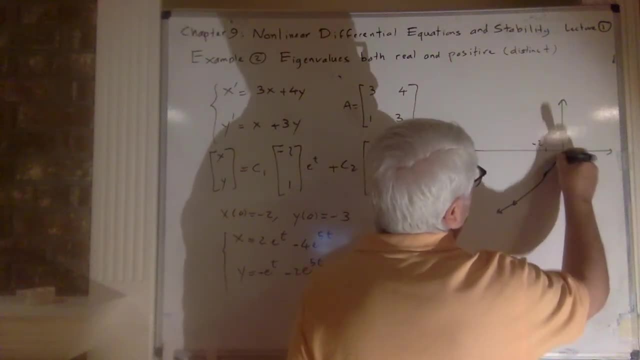 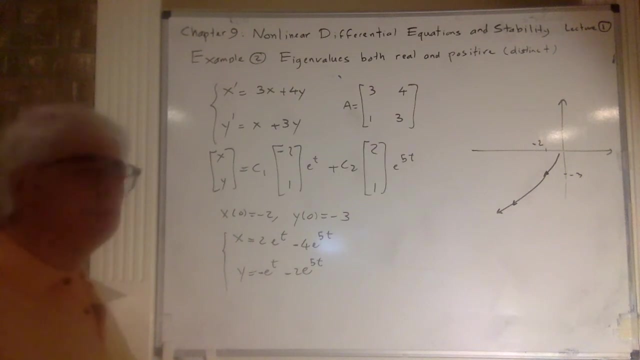 this way, way, but never reaches zero. in fact, If you graph it for negative time, it never reaches zero again. Zero, zero. And for the same reason, And also the critical point is the same: zero, zero. For linear systems, well, this matrix is not singular or the determinant. 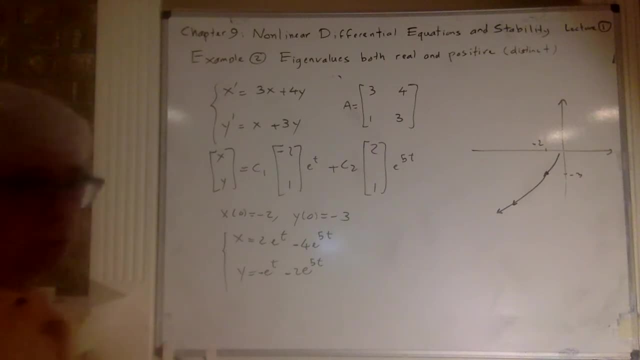 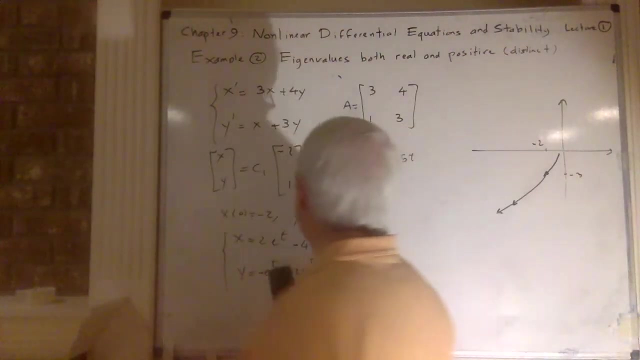 is not zero, we will have what? X zero, Y zero. that's the only answer. So for linear systems, that's the only critical point, and no trajectory reaches that zero, zero. Now let's graph these two separately, So that was like parametric plot: the X and the Y. 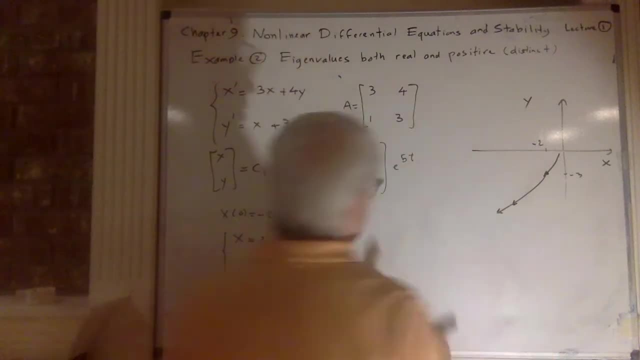 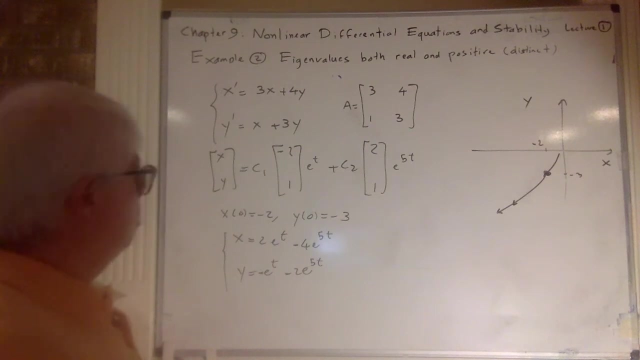 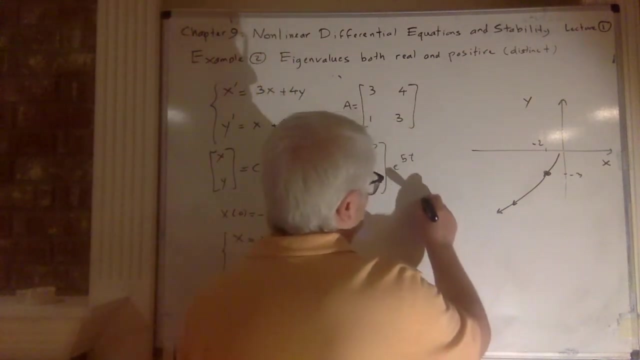 was the parametric plot. Parametric plot of this gave me that and the parametric plot starts here And if I plot them separately, they're just functions of time, Just the functions of time, And they look like this. In fact I plotted them. In fact both are. 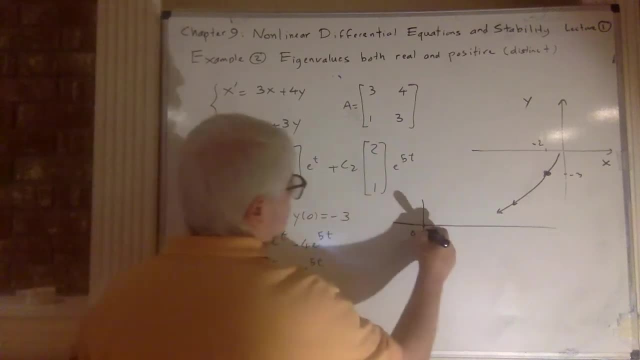 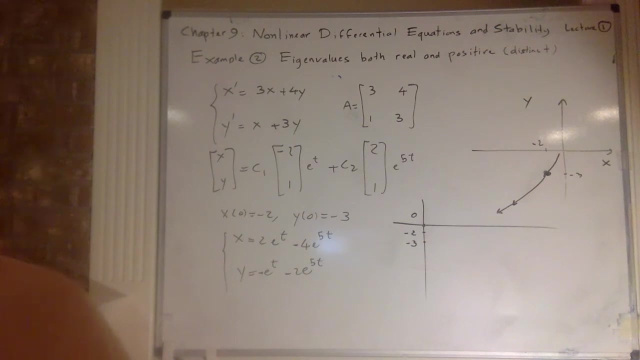 negative. So now this one, X, starts at negative two. So let me put zero here. This one starts at negative two, this one starts at negative three, And I had this picture here. Negative two goes like this, And this one goes like this, And this one goes like this, And this one goes like this. 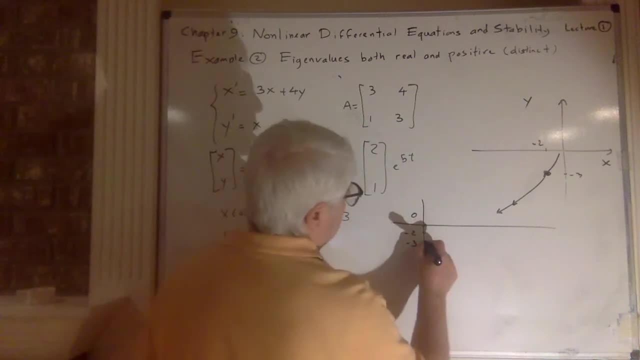 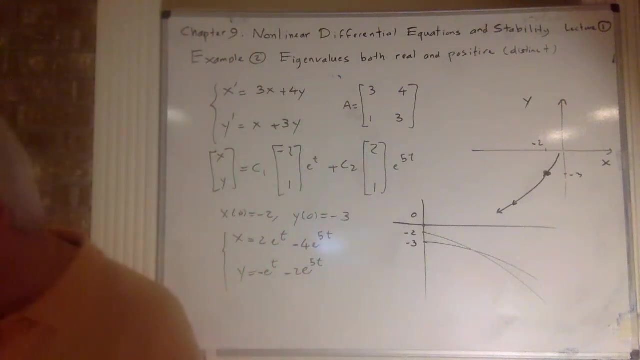 the negative 3 goes like that, so the negative 3 goes like this, the negative 3 goes like this. okay, And in fact I found the exact in this time, I found the exact for time. this is time, and this is the x and the y. which one is the x? this one below this, the y, in fact. 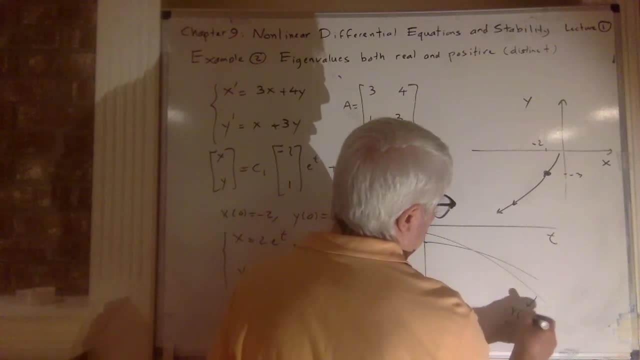 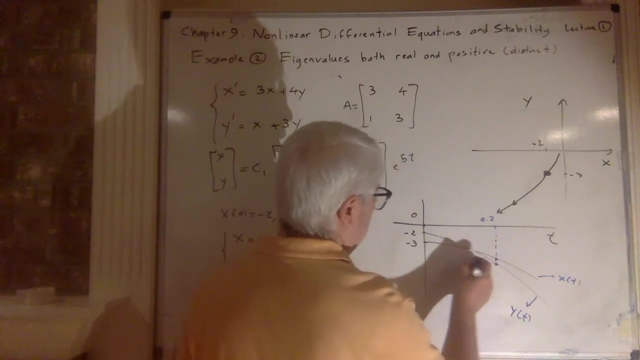 this one is the y and this one is the x. And for point 2, in fact I found: for point 2 I found minus 6.65, minus 8.4.. So for point 2, I found this and this. so this is a point minus 6.65,. 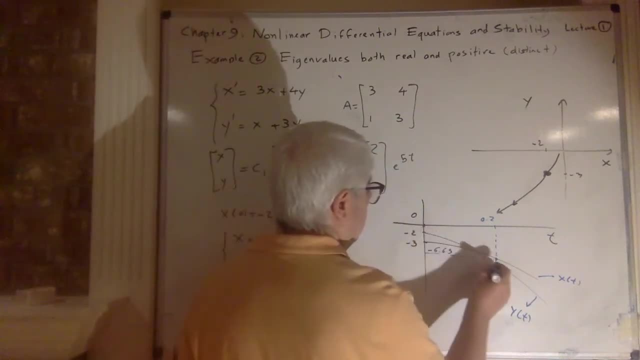 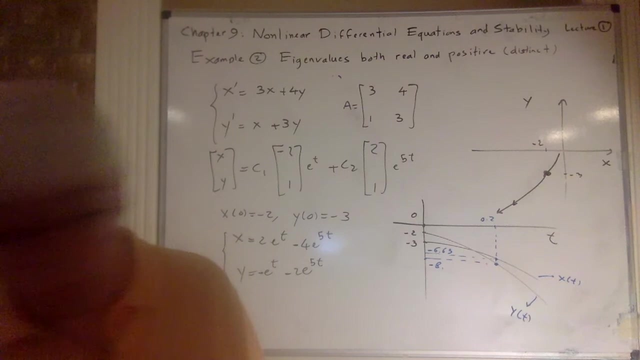 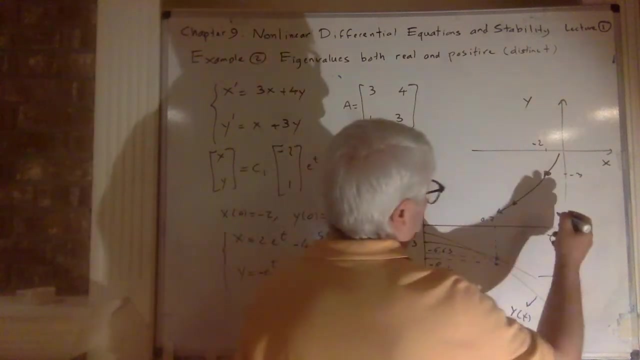 and this is a point minus 6.65.. So this is the x and this is the y. so x is 6.65 and y is minus 8.4, minus 6.65, and that's this point here. So this is the y. 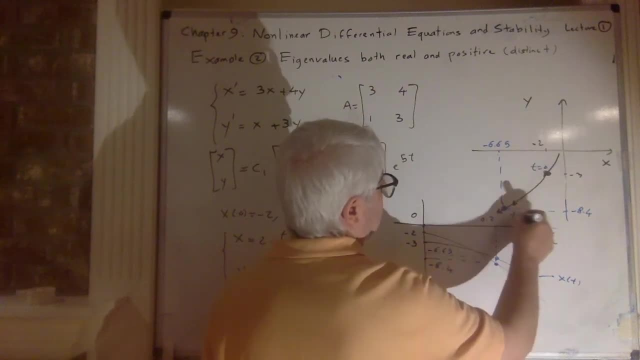 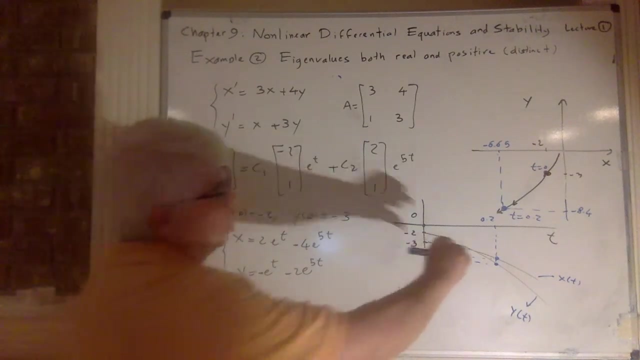 So this point, this is time 0,, this is time equals 0.2.. So time equals 0.2, it is at this point And you can see that it just goes to negative infinity. This also goes to negative infinity. negative infinity, right. 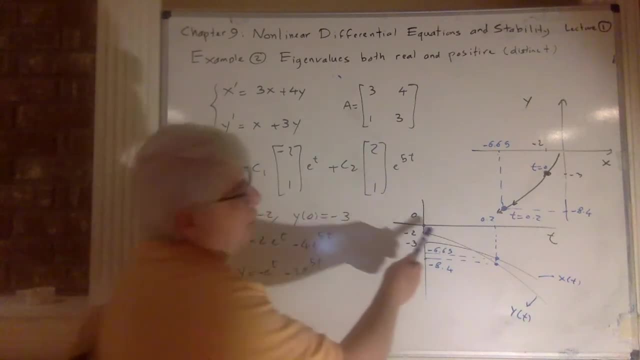 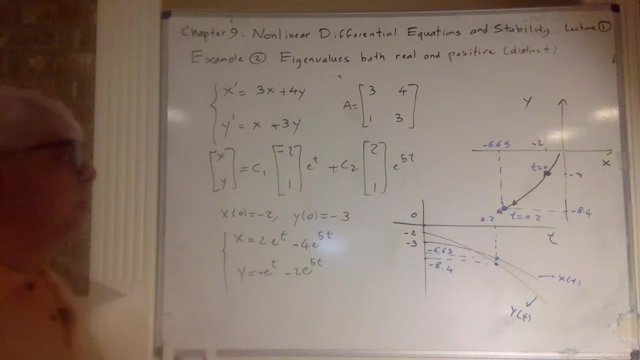 Both x and y go to negative infinity, and separately you can see that they are just diverging. So this situation is, in fact, when it's diverging, It's divergent And we say that this is unstable, unstable, unstable. So let me summarize here for these two examples: 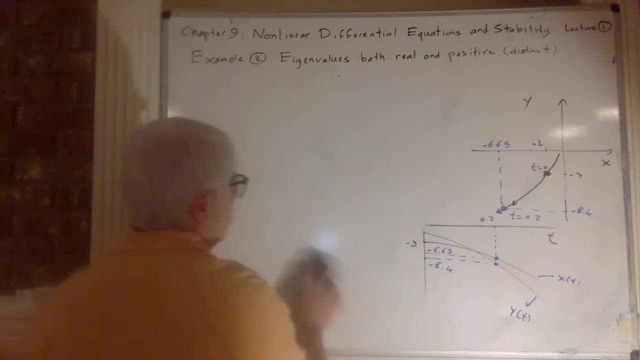 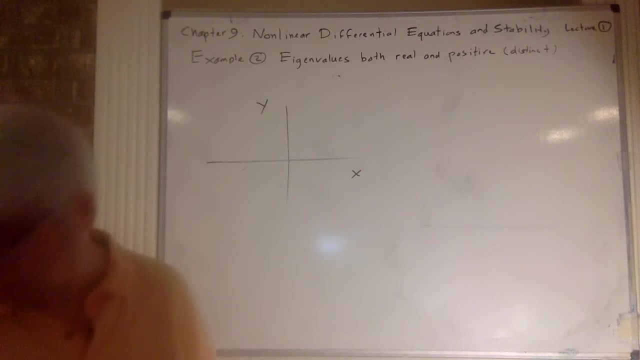 If I give you the phase, the x, y, if I just graph some streamlines, the streamlines should: yeah, they look like this. So the streamlines will be like this. So this way, this way, this way. 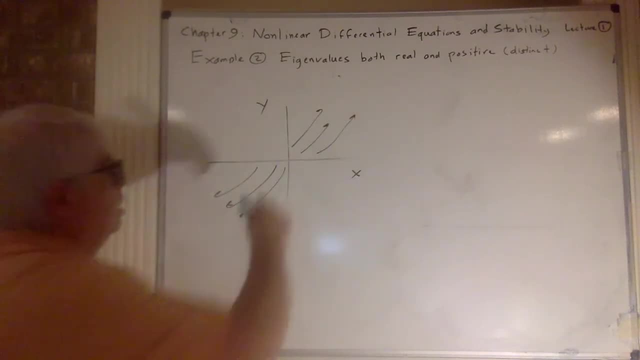 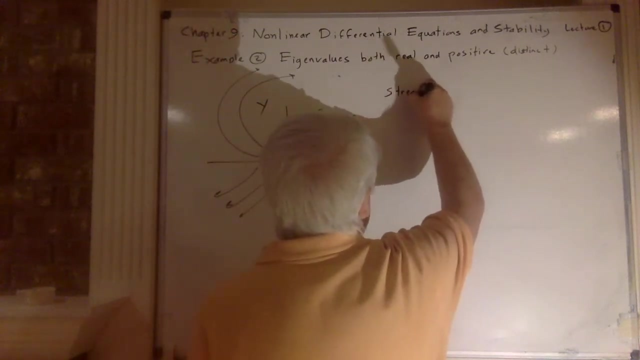 They go this way. And if you start, here it goes like this, And it goes like this, And it goes like this, And here it goes like this. So you can graph this thing on mathematical or look for multiple And, if you don't remember, photograph it as a stream plot and give the what was that? 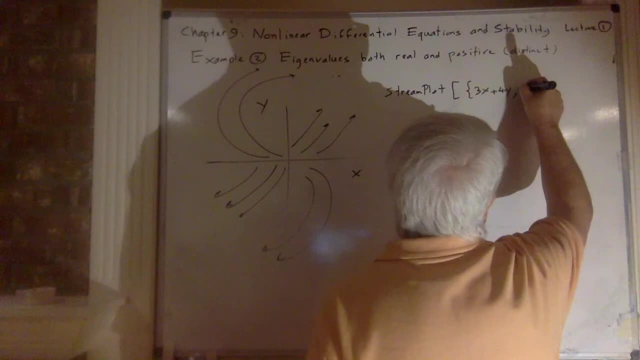 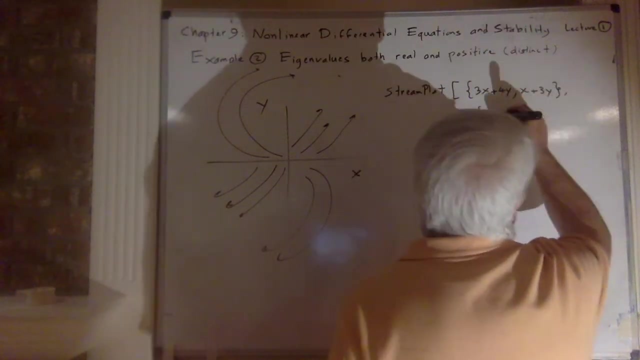 3x plus 4y, comma x plus 3y And you can give x. x goes from- I don't know- minus 5 to 5. And y goes from minus 5 to 5. It doesn't have to be the same. 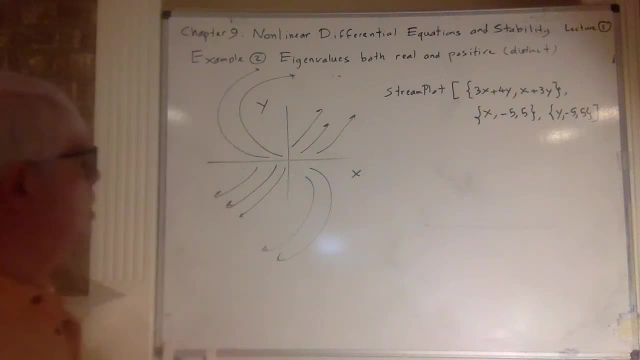 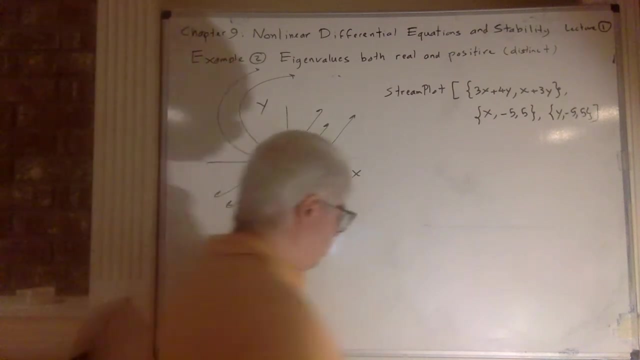 You can do something like this on mathematical and you get this stream plot, And one of them was our solution, the one that starts at negative 2 and negative 3.. Okay, And you can see that they are just going to infinity. Wherever they start, they go to infinity. 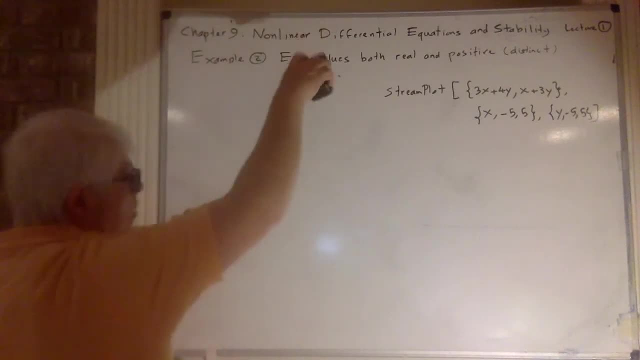 But it depends on where they start. It might go like this way, infinity like that, infinity like this way, and so on. Okay, Now the other situation. I have to summarize. So lambda 1 and lambda 2 distinct Distinct. 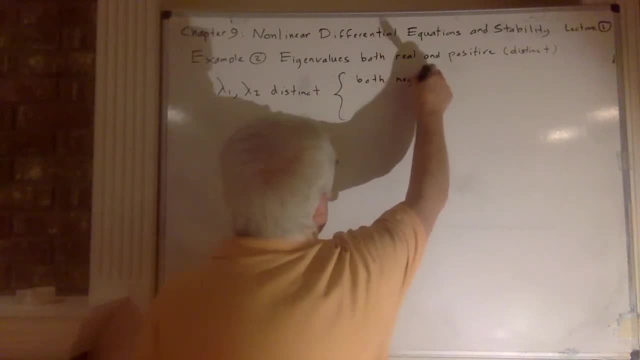 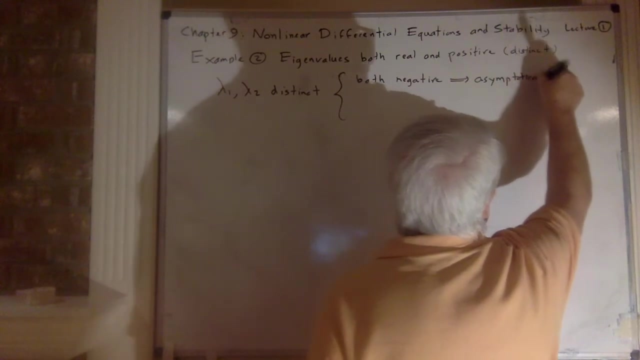 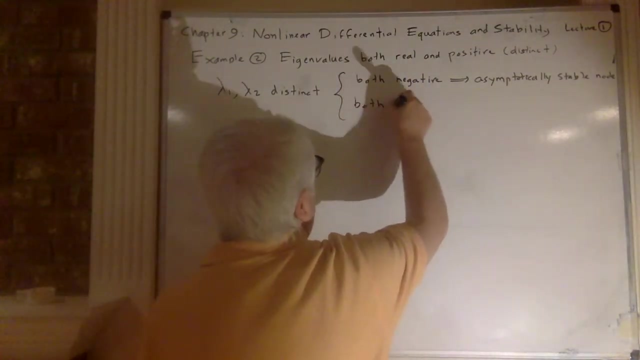 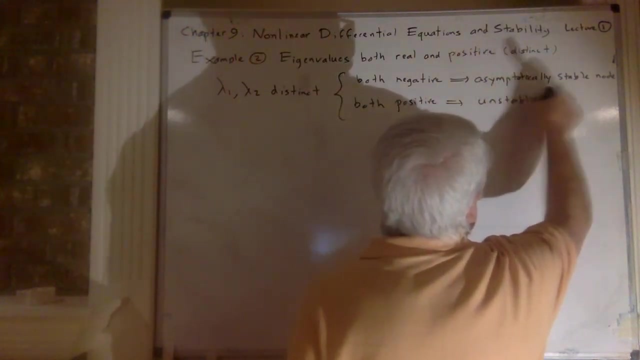 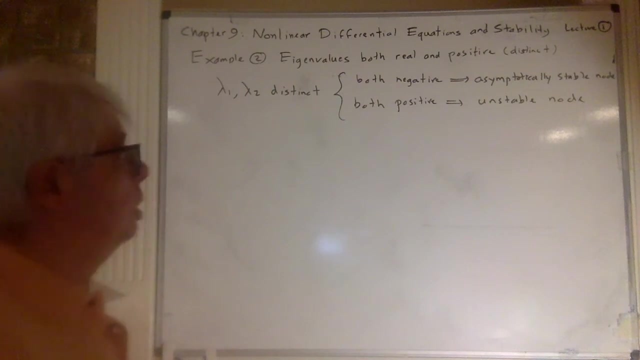 Both negative But, as in totally stable node, Both positive, Unstable. So if they are both positive, as you saw, the two solutions, whatever they are, they just go to positive, negative, infinity. It depends on the situation And that is not acceptable, at least. 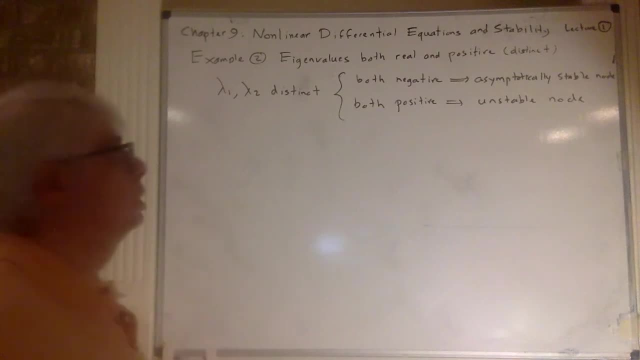 If that is the system, it will break Boom. So these are the two situations that we have, distinct and not the same. Well, let me find one that has two eigenvalues. Well, I will explain then. So what happens if they are distinct? 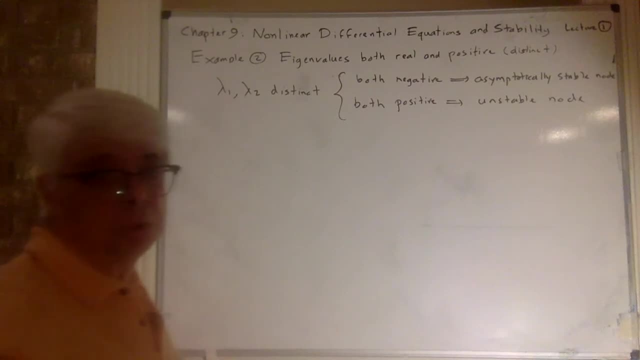 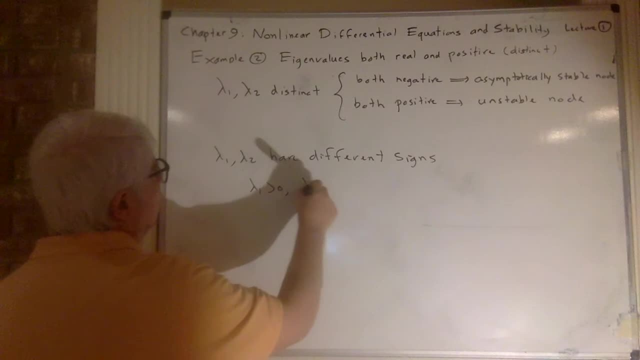 So let's say lambda 1 is bigger than 0, and lambda 2 is less than 0. So solutions are linear combinations of these two right. Solutions are linear combinations of e to the power lambda 1t and e to the power lambda. 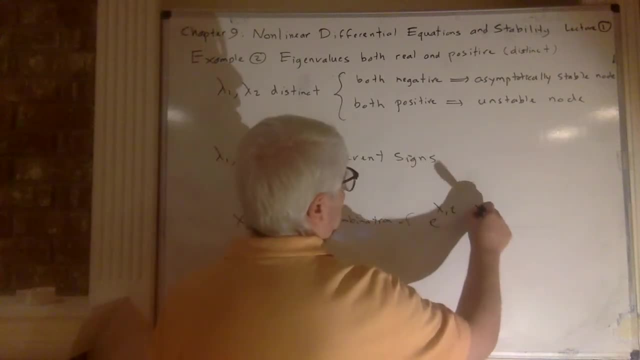 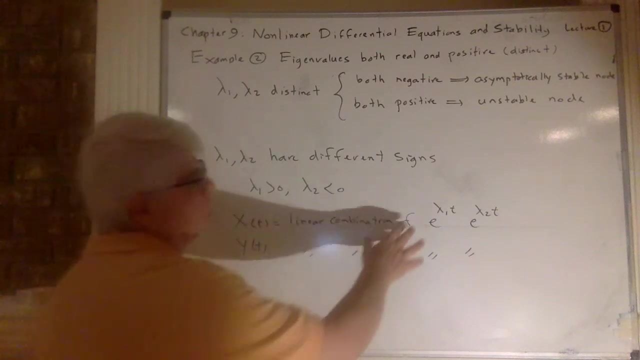 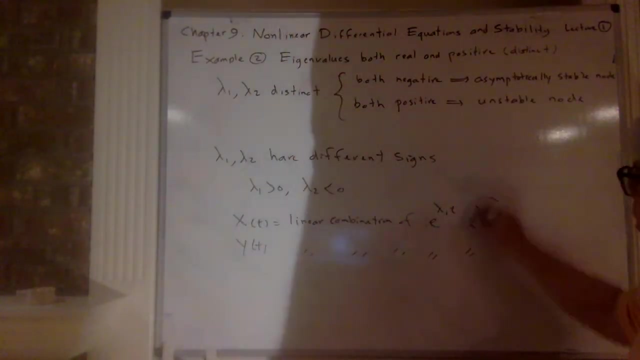 2t. Okay, Okay, Okay t and y t, also another linear combination of these two. Well, depending on the linear combination, depending on the positive, negative, whatever that is, this is what happens When this is less than zero. so it is e to the power minus 5 t, So this goes to zero, basically. 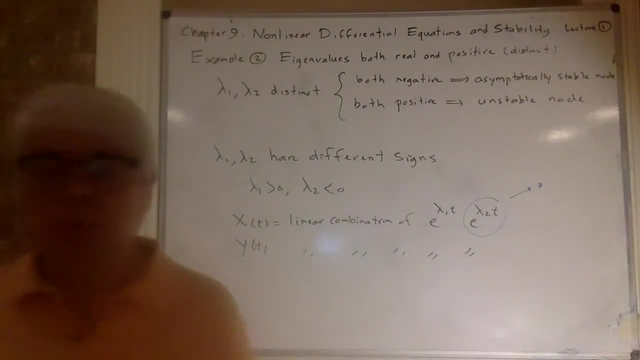 right, As time goes to infinity. this one goes to zero. What happens to the other one? This one goes to infinity. right? So I have something that goes to infinity, depending on the coefficient of that linear combination. It might be negative infinity or it might 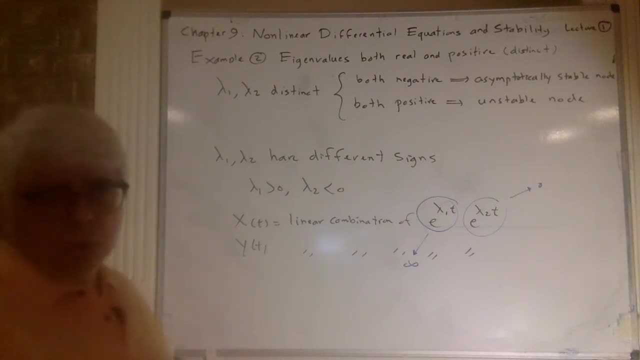 be positive infinity. But the other one is what The other one is? basically, if t gets larger and larger, that one goes to zero. So this one basically is talking: say And unless, unless the coefficient of this one is zero, okay, So what happens here is that as time 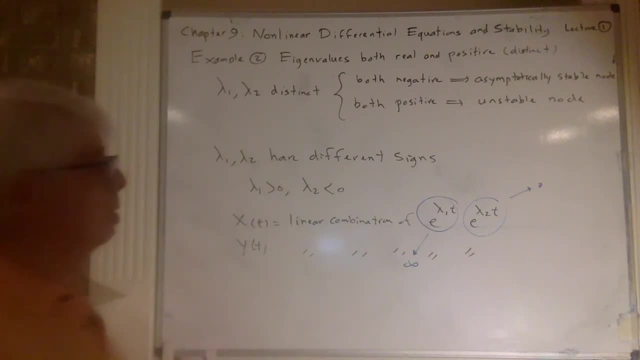 goes if, when time gets larger and larger, depending on the situation, we might have stable or we might have unstable. So this situation depends on where you start or what coefficients you have and things like that. So I will give you a much nicer example in: 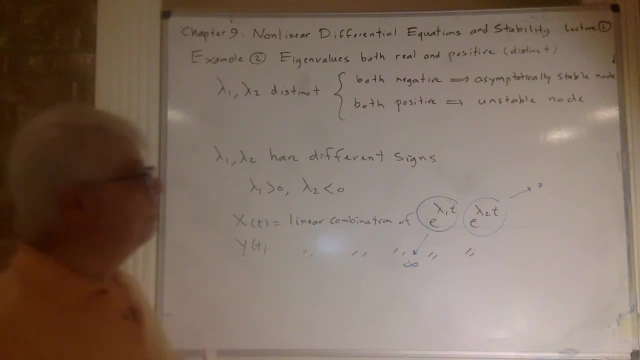 the next lecture And then I will graph everything. But this one is like what we call a semi-stable situation, So I will write down an example for you. I don't want to just jump on some example on the fly And then I don't know if there are two or different signs, So I should hook up. 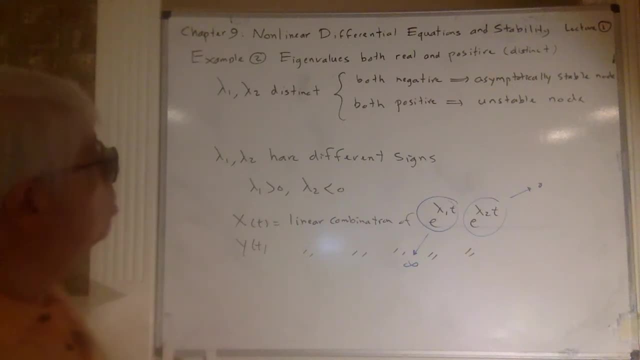 something for you. Okay, so that was lecture number one and the two situations of stability, And the first one I'm going to show you. I'm going to show you how to do it, And then I'm going to show you how to do it, And then I'm going to show you how to do it, And then 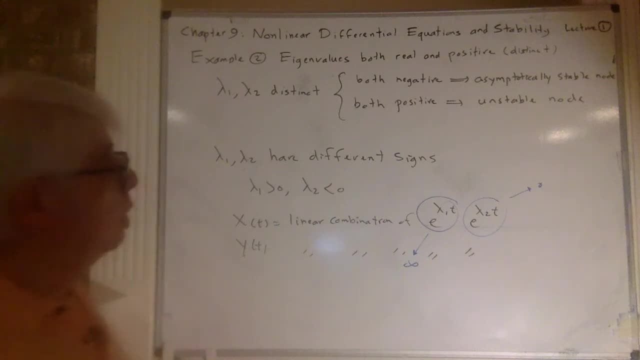 I'm going to show you. I'm going to show you how to do it. So the first one, both negative- is desirable. So if you are designing some system, you have to be careful to design it so that the eigenvalues are negative, for example. Now situation: